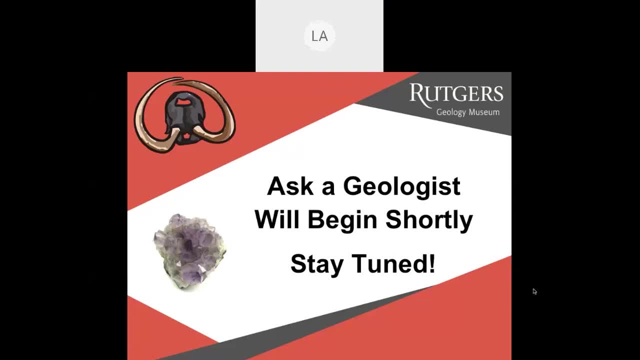 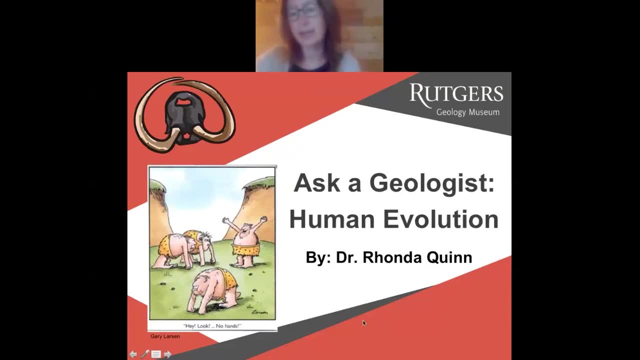 Okay, thank you. So can everybody hear me? We are going to talk about human evolution today, And this is a bit of a joke, but when we talk about when we became bipedal, that's a bit of the time period that we're looking at And we're going to think about all the 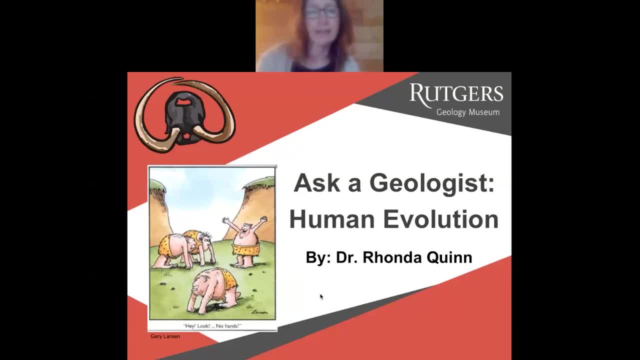 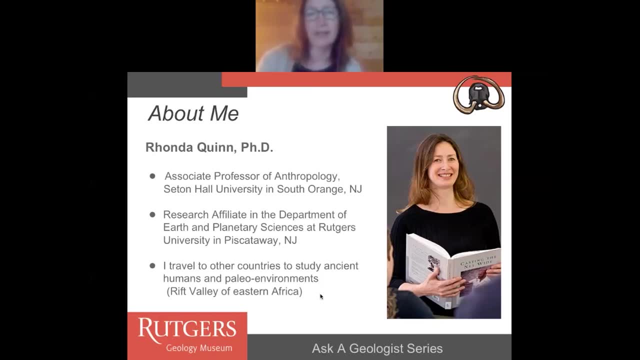 ways we try to reconstruct this from the past, And so let me tell you a little bit about myself. I'm an associate professor of anthropology up in South Orange, a little bit north of Rutgers, And I'm also a research affiliate with the Department of Earth and Planetary Sciences. 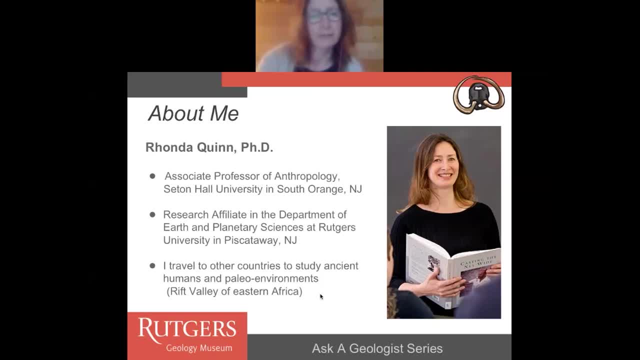 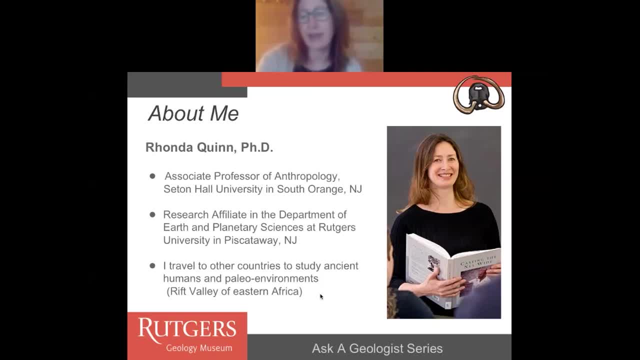 a big joy for me, especially in the Rift Valley of Eastern Africa. Unfortunately, I haven't been able to take my kids there yet, but I will soon enough, when they're old enough to go. And so a fun fact, and I'll talk about this. 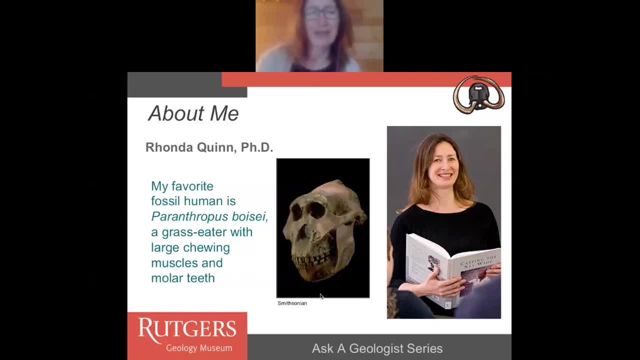 this early human a little bit later, but my favorite fossil human is Paranthropus boisei, which is its name, And what's so interesting about this one is that it was a grass eater, which is very unusual for humans, And it had really large chewing muscles and really large back teeth and older teeth very large. 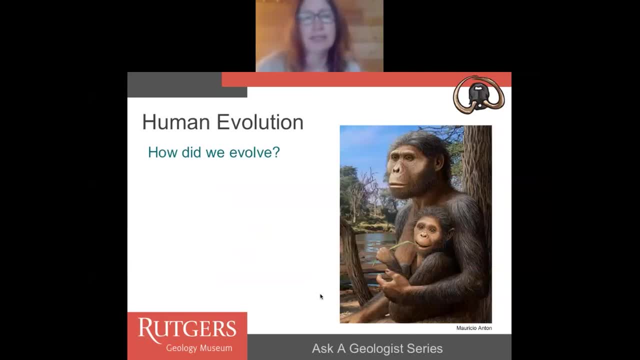 So let's think about human evolution and kind of, how did we evolve? It's a big picture. It happened over many millions of years And when we think about evolution it's probably most important, at least when I think about how to understand the past. 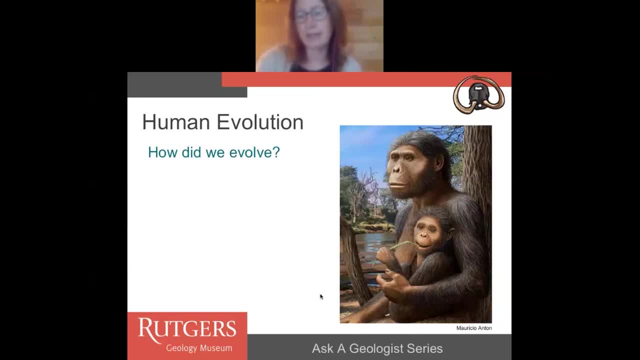 is to not just understand the organism that lived in the past, but try to make a link to the kinds of environment that the animal lived in, because those environments would have shaped human evolution. And so when we think about what kinds of environments, we want to reconstruct the past. 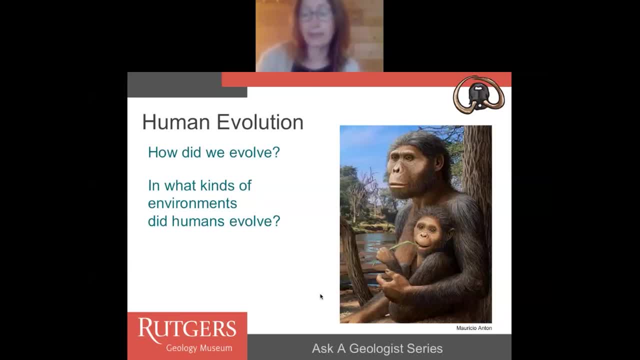 in what? was it a forest, Was it a grassland? Was it hot? Was it cold? Some of the things that we think, think about in our natural environments today, because it's going to be certain traits that we think are important to humans and what defines us as humans were selected, meaning that they were. 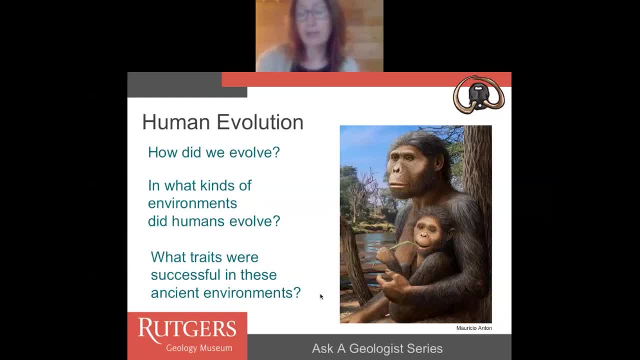 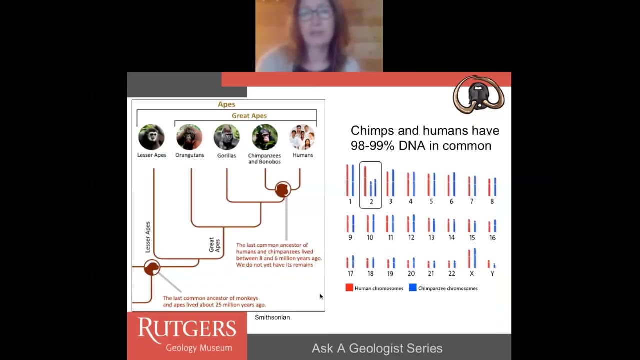 successful in these ancient environments. So we like to make the link between the organism or our ancestor and the environments that they lived in. So just to get us started to think about human evolution, it's really useful to first think about where we kind of sit in the animal kingdom And our closest ancestors are the chimpanzees. 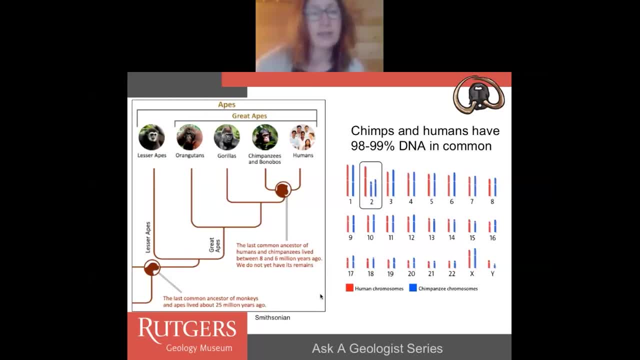 And so if you look at this, what's called a phylogeny on the left side of your screen, that tells us that we are a part of the great apes, We would be considered a great ape, and what's interesting is that chimpanzees and humans are very closely related, And so 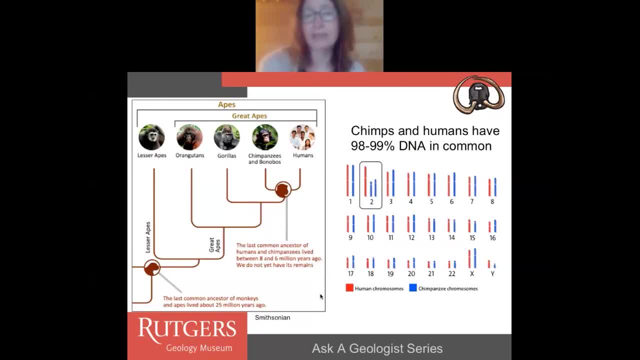 with modern humans, living humans and living apes today. we have sequenced their DNA for the building blocks of their life, And so we know. if you look at the picture on the right, you can see that chimps in blue and humans in red are very close. They share actually a lot of DNA. 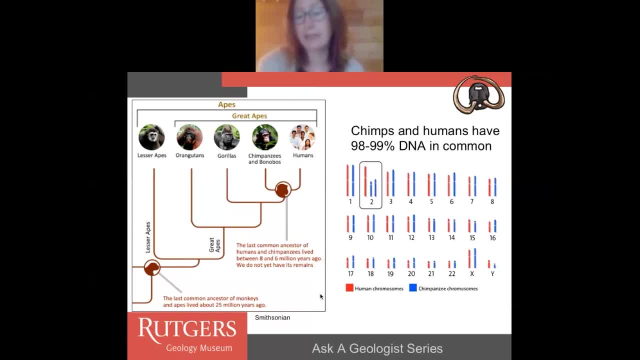 this was not something that anybody expected, but we realized that chimpanzees and humans are actually closer when it comes to how much DNA they share in common than, say, chimpanzees are to gorillas, And that was one of the eye-openers, that was one of the surprises we thought, because we thought 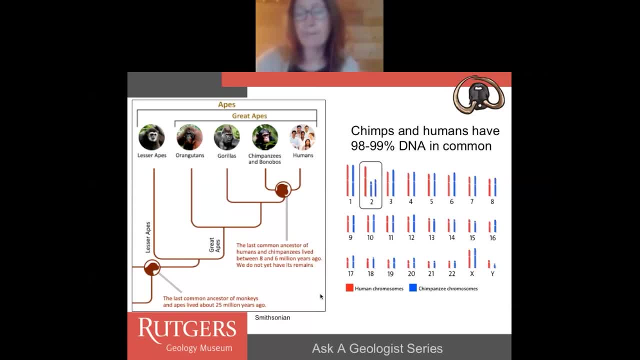 chimpanzees and gorillas. both being apes from Africa, we thought they would have been more closely related, But as it turns out, they're not. They're not. Chimpanzees and us are very closely related, And so we can see that this split happened some. 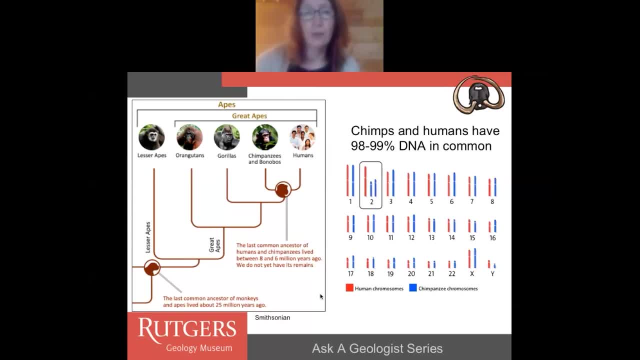 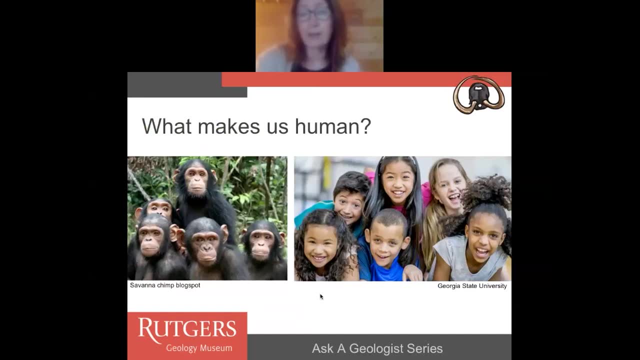 time ago and to kind of understand what makes us human and what makes us, what are these environments and what was our evolutionary process that we went through to be different. it's kind of a it's a question about this kind of 1% of DNA. This 1% of DNA makes a big difference. between chimpanzees and humans, And so we can see that this split happened some time ago, and to kind of understand what makes us human and what was our evolutionary process, we also have to look at these ability to share andSOF. 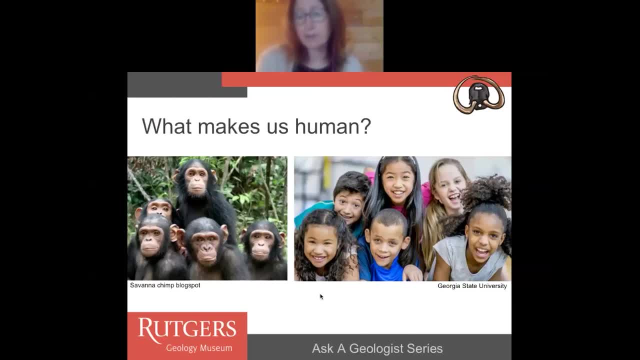 So they're really sympathetic to chimpanzees and us. We know we have very complex social systems. we know we have very high intelligence levels, a very large brain, a brain, on average, that's three times that size of a. We know that we have a much bigger body. 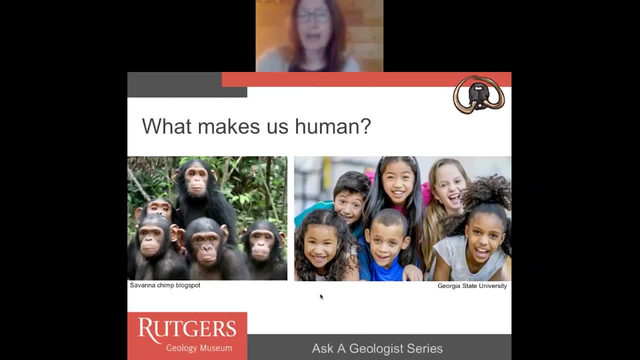 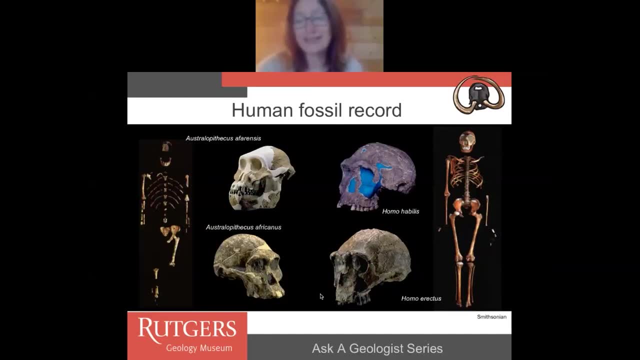 and we know we have language. But when it comes to actually thinking about this in the fossil record, that's when it becomes a little bit harder, because we're reconstructing something from our memory with our culture, And so that's what we're trying to do. We're 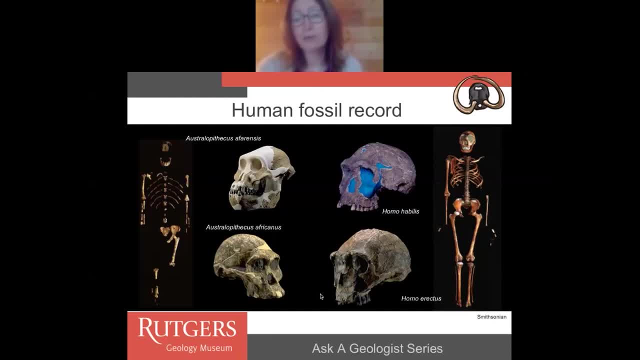 fossils And so much of what's preserved in the past doesn't necessarily give us a direct idea about intelligence. let's say We can identify brain size, but it doesn't tell us about how the brain works. We can look at body size, but it doesn't tell us all about the soft tissue We have. 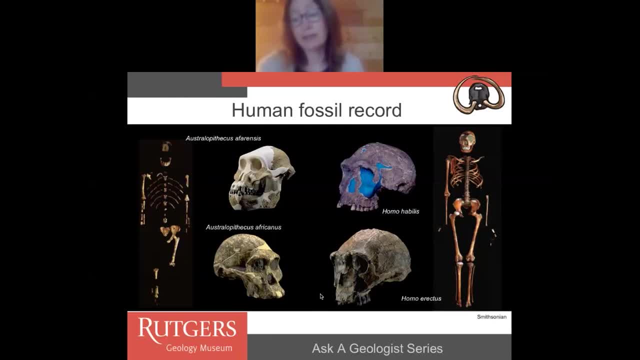 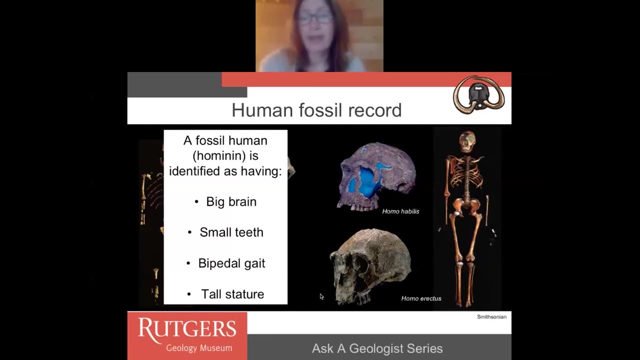 to make guesses, Well, we have to make inferences based on what we see, And so, when it comes to the fossil record, what we can say is that there are some things that all humans, we think, share in common, and these are things that we have today, compared to, say, chimpanzees. 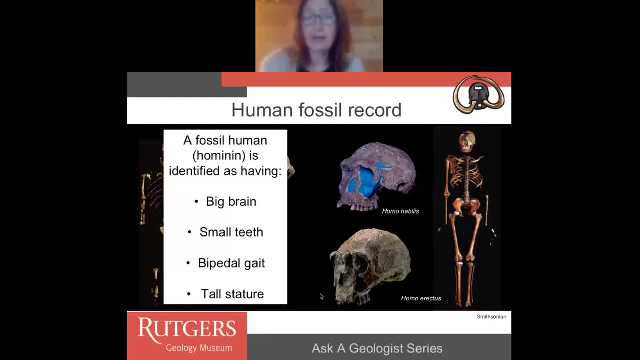 And so when we find a fossil, when we pick up a fossil, we typically look at some features from it to say like, oh, it is a fossil of us and it's on the road to us. It's not something that is. 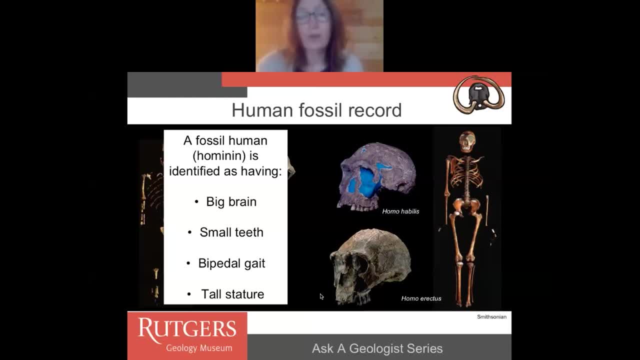 likely an ape or a non-human ape, And so one of those things is a big brain. How big? That's a good question. We'll talk about that in a minute. We do see smaller teeth. A lot of this happens, not right away, but we all are characterized by having, you say, a reduced dentition. We get a. 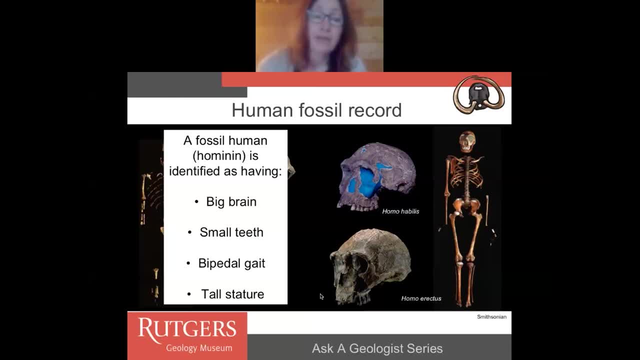 flatter face with those small teeth. We have a bipedal gait, We are, we say, habitual bipeds or we're always walking on two legs And everything about our anatomy, both the hard tissue right, both the skeleton and the soft tissue like our muscles, everything is basically right. 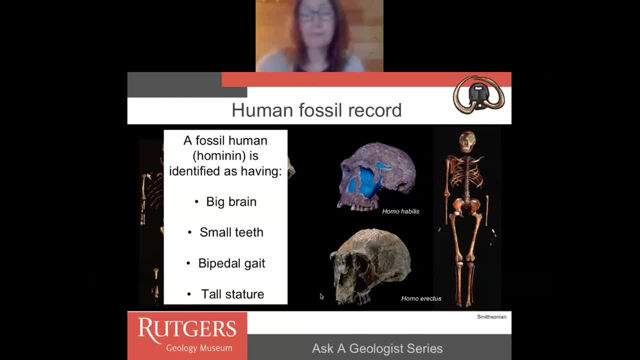 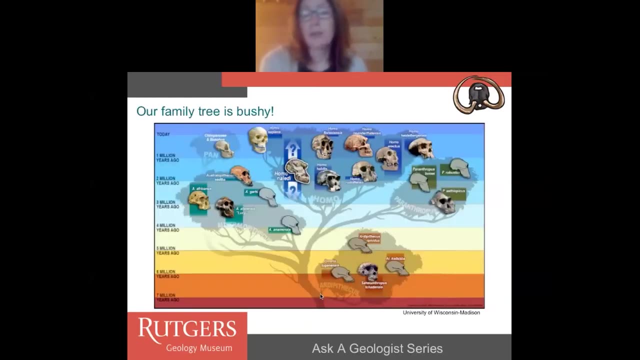 configured in a way that we are always bipedal And that we also are tall compared to other, especially other apes, And we can see this with our long legs and that may be related to our bipedal gait. So when we think about the evolution and the split probably between six and eight, 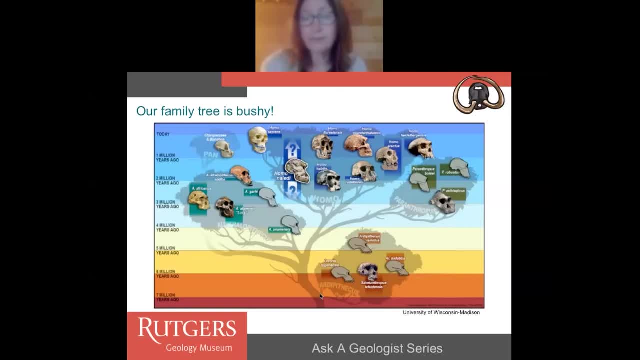 million years ago. what does our family tree look like? And, as it turns out, our family tree is very bushy. It's not as if it's one lineage that gives rise to another. What we think is that we have lots of different paths. We have lots of different paths. We have lots of different paths We have. 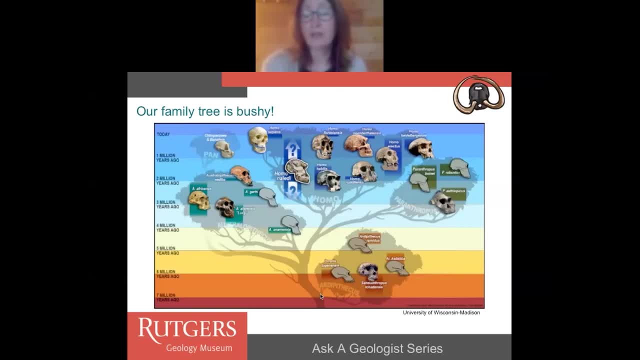 lots of different ways that the- let's say, the human family tree experimented with things that worked and what didn't work. Some went extinct, Some kept going, And what we think is that there's also a difference in the amount of time that things show up. So, for instance, we think the split between apes and humans. one of the earliest features that showed up was being bipedal. That's about six million years ago at the earliest and it bumps up to about four million years ago. So being a biped and being a habitual biped shows up. about then Having small teeth. small teeth- 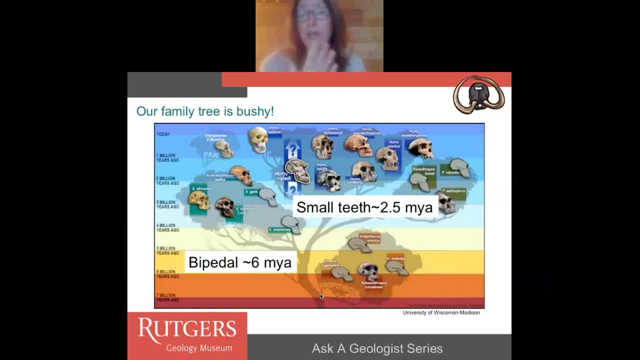 closer to what we have today. in these flatter faces we don't see that really happening. until about two and a half million years ago, The MYA stands for millions of years ago. Now we don't get tall. until about 1.8 million years ago, We don't. 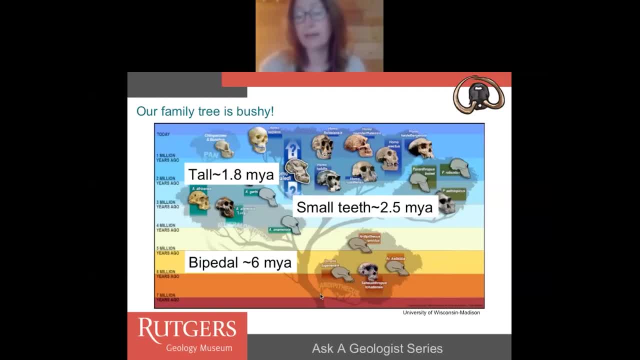 see kind of the body configuration with the long legs and the narrow hips and basically the tall stature until about 1.8.. And then, finally, the big brain. We see glimpses of the big brain, but the big brain that we have today really shows up at about one million years ago, So it's relatively 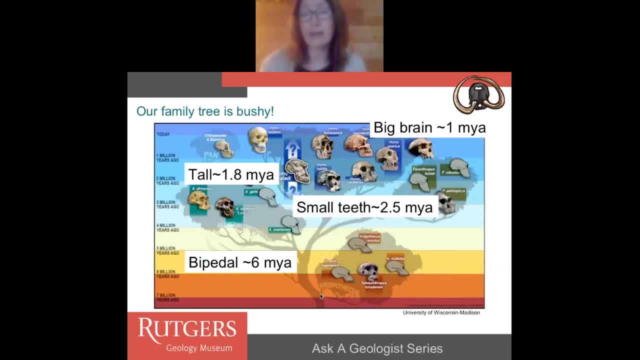 late in our evolutionary history that we see that. And again we're kind of relating the size of the brain to intelligence. But that's something to work out that there's different types of intelligence. Now we can see that kind of traits evolve at different times And so what were kind of the environments? 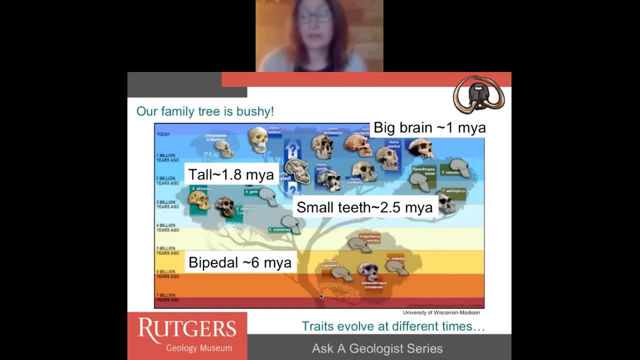 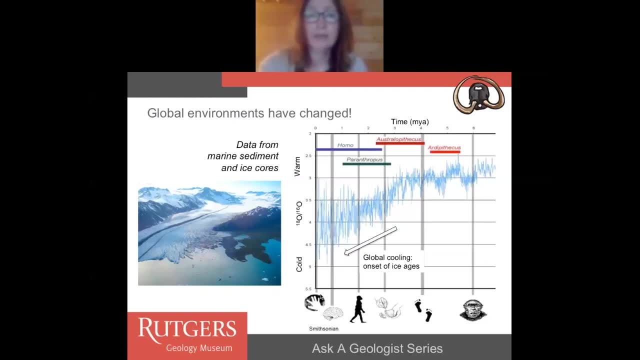 during this time period, because this is a long time of Earth's history, of going back to about six million years ago. what do we see And what we know? and a lot of the types of data that are generated are generated in places like the red grid. 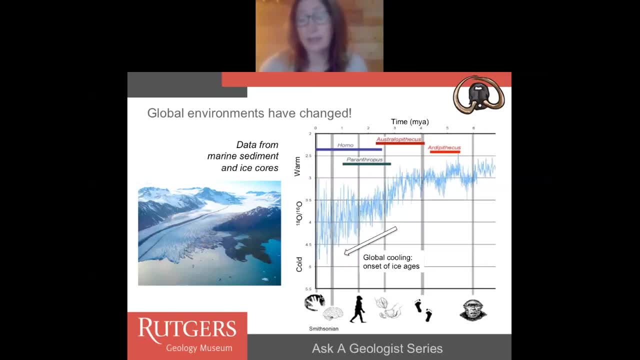 So this is the data from the US Department of Energy's Department of Earth and Planetary Sciences, and Dr Adamo is one of the people who generate these types of data. So, from marine sediment cores and even ice cores, we have an idea of what global climate, but also global environments, look like, And so, during the 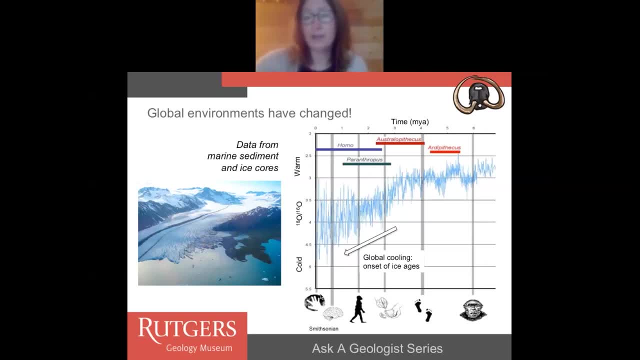 time when you can see this squiggle. this blue squiggle is actually measured marine cores And really the data from these studies. it's a proxy of temperature, And so what's happened about over the course of about six million years is that we see the globe is cooling, So we have the onset of the ice ages. 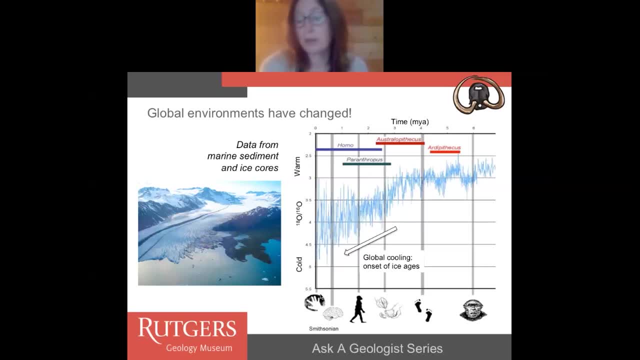 And during this time period we also see a whole host of different species coming up and evolving. Now most of our evolutionary history is actually in Africa. So from about six million years ago to about two million years ago- that critical time period, including the rise of our genus- 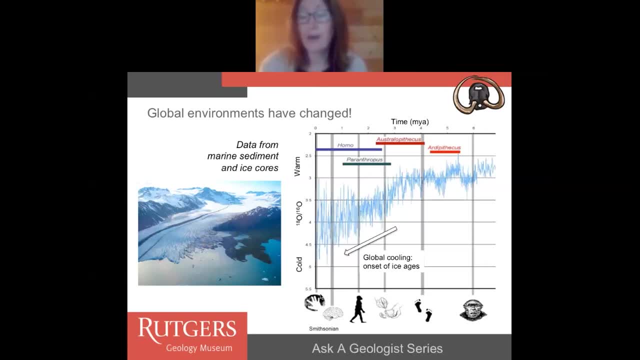 genus Homo happens in Africa, So a part of what's going on globally. we also want to think about what's happening to the local environment in Africa And what we see across this time period is there's also a big shift, So global temperatures are changing, but also vegetation. 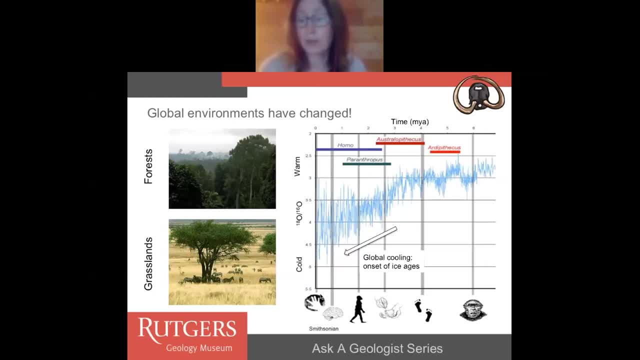 is changing, And so what we see across this time period is there's also a big shift, And so at the equator, in both actually Eastern Africa, but also Southern Africa as well, we have more dense forest cover about six million years ago, And what we see is through time, 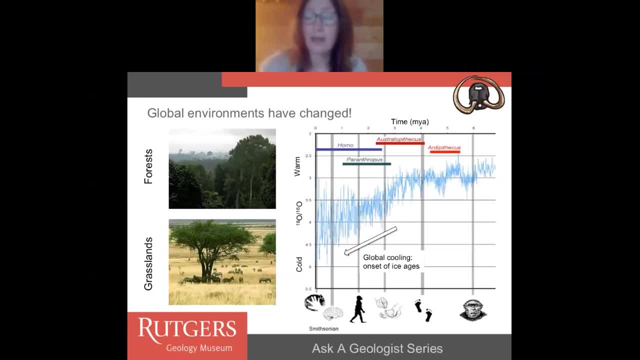 a breakup of those ecosystems and an expansion of grasses, And so these are tropical grasses. They feed lots of animals. Think about the zebra that you see there in the picture today, Also the antelope. It supports a lot of organisms And it's the rise of these grasslands that is. 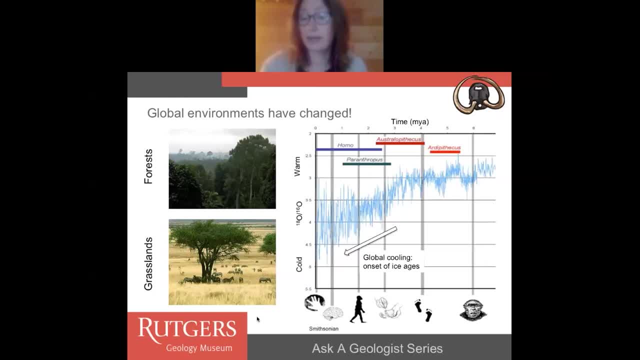 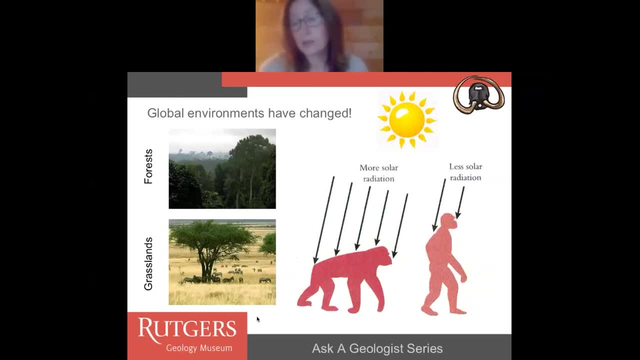 coincident with the rise of a lot of our ancient species. One of the ideas is that, with this change in a forest cover and having a tree cover that's very dense, and once we break that up and we basically have trees that are still present but they're. fewer and farther between. we get more solar radiation. And one idea- and there's many ideas about why we became bipedal, but one of the ideas early on is that the beginning of this breakup then gave us more solar radiation. We were exposed to more solar radiation. 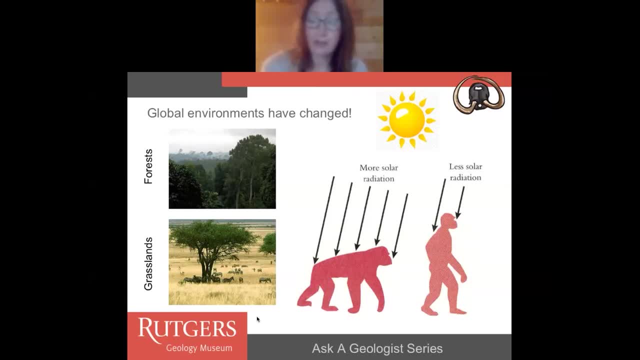 And so our lineage- not the apes, but our lineage- started to venture out and may have been foraging across these or eating across these landscapes, And they were selected to be bipedal because it actually exposed their body to less solar radiation. And so, as temperatures are getting, 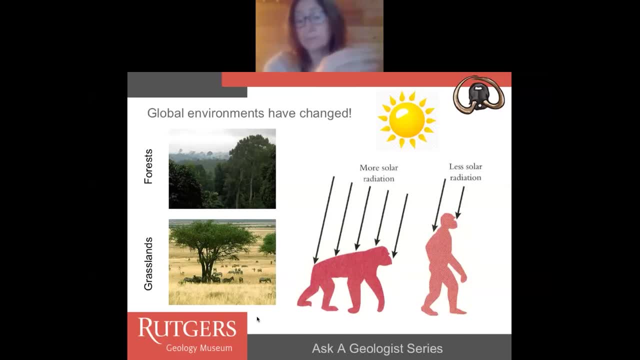 really hotter and drier because of the less tree cover in the tropic. this would have allowed a little bit more cooling of the body, And so it was really about how to stay cool And still forage your food, And so being in a bipedal mode may have been one of the reasons. 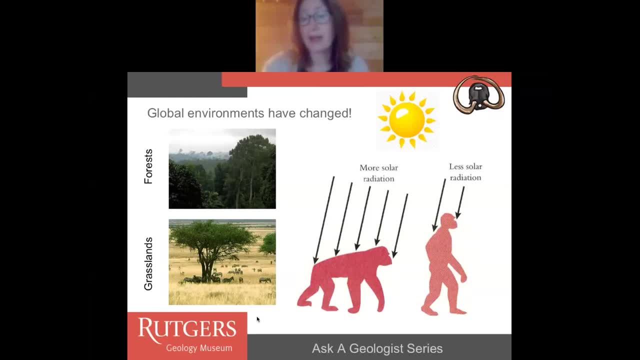 Another reason is that we see that this type of locomotion, especially for distances, actually gives us a lot more calories, And so, for instance, if we were walking the same amount of distance as a chimpanzee walking on a horse, we would actually burn fewer calories. So it may have been not only the solar radiation. 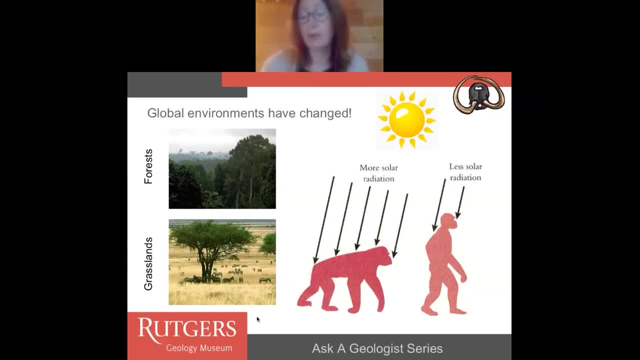 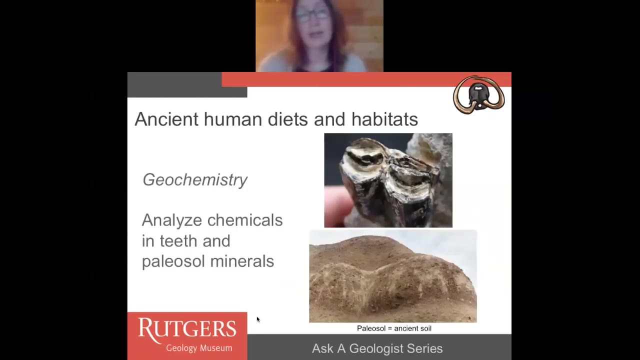 but the distances we were traveling were important in these landscapes, these broken up grassland landscapes. That was the environment that selected for us to be bipedal all the time. Now, my piece in this is that I want to reconstruct both the diets of ancient humans. 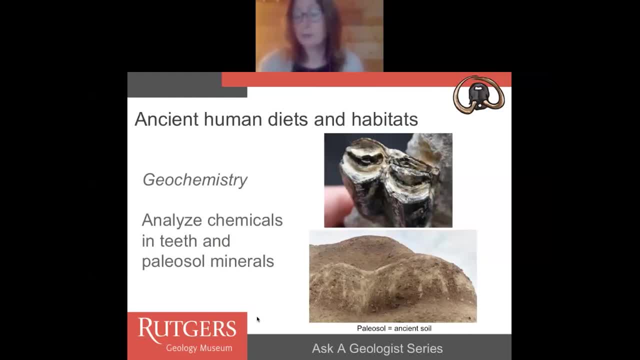 but also the habitat, Because we know that organisms do compete over different food resources and environments. And so the idea is that to bring evidence from what does the habitat look like? Was it a grassland, Was it a bushland, Was it a woodland or even a forest- And bring 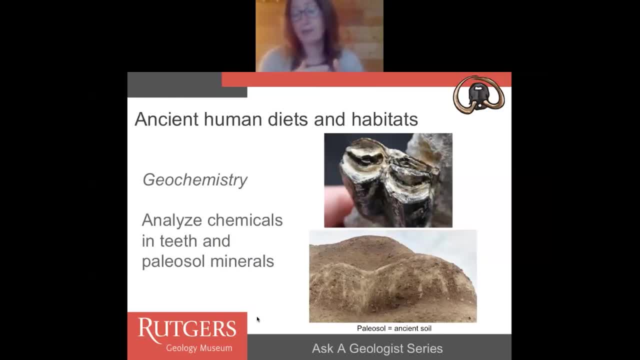 that to bear with the actual diet of the human. And so how would those basically? did they mash up, Did they match Or were they unmatched? And so, with geochemistry, and this is one approach that we use over in Earth and Planetary Sciences, 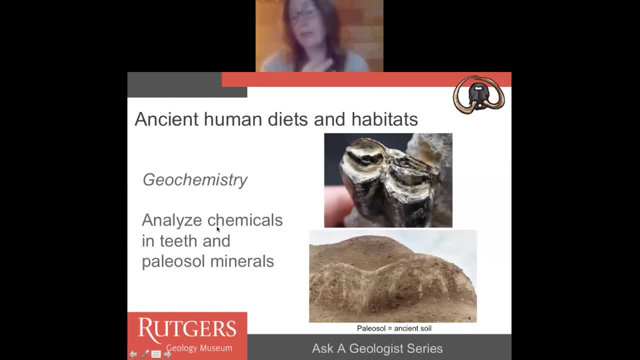 at Rutgers is to analyze the chemicals in things that preserve in the fossil record. One of those things is teeth, And so we look at teeth of other mammals, we look at teeth of humans, and then we also look at things that preserve in the past, like this ancient soil. 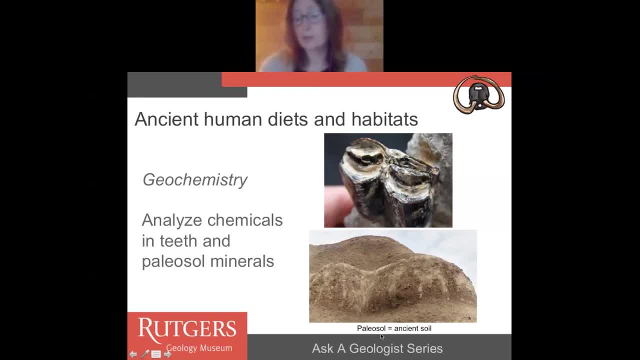 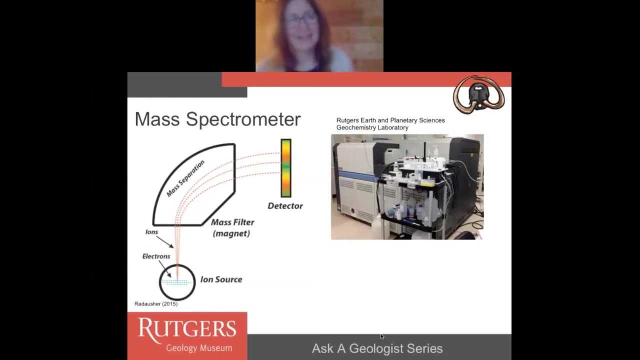 So the paleosol is just another word for an ancient soil, So we can actually look at the minerals that are preserved within there and get an idea of what the environment looked like, And so we get to use some pretty fancy equipment to do it. One method is that I use with 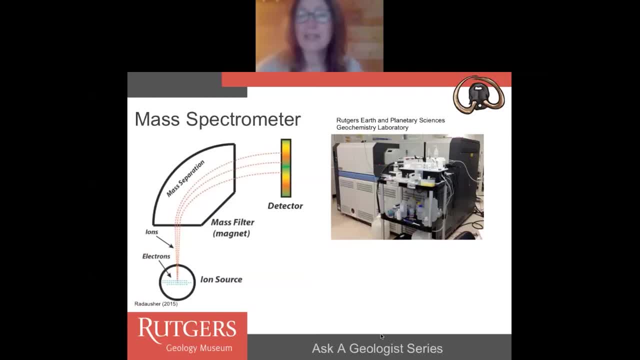 geochemistry is what's called a mass spectrometer, And you can see a picture of this mass spectrometer. We have several, but this one in particular is at Rutgers Earth and Planetary Sciences in the geochemistry laboratory. This is where we separate out different elements based on how heavy they are. 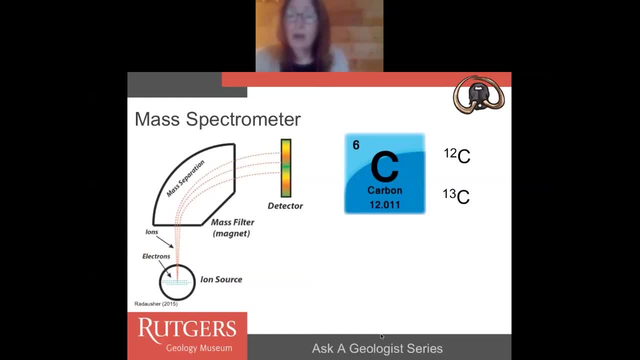 So, as an example about one of the ones we look at is carbon, And so carbon is- and you might know this if you're taking a chemistry class, if you've taken a little bit of the science classes- that you see that carbon on your periodic chart has. 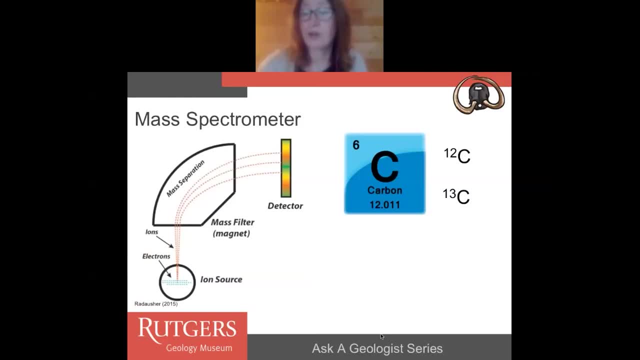 the carbon that we see mostly around the Earth is carbon 12. It has a mass of 12. But in the natural environment there's also a heavier carbon called carbon 13. And if it turns out, when we measure these two, we get an idea. say, for instance, from one of those paleosols we get an idea of what the 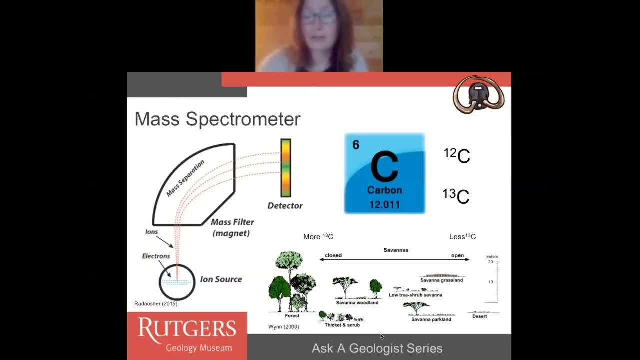 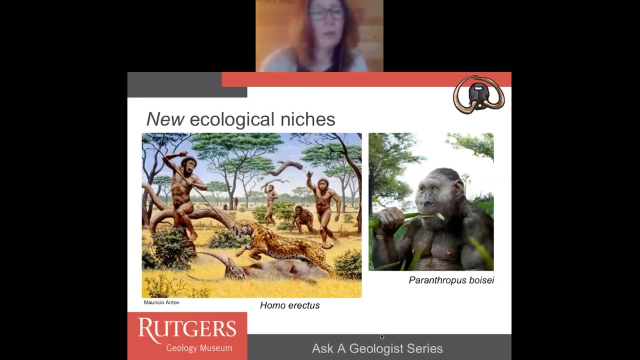 environment looked like. So what we see is that forests have more 13,, more of the heavier carbon, whereas the grasslands have less of the carbon. And so what we see is that when we look at the diets of animals, when we look at the natural environment, we see that this bushy tree 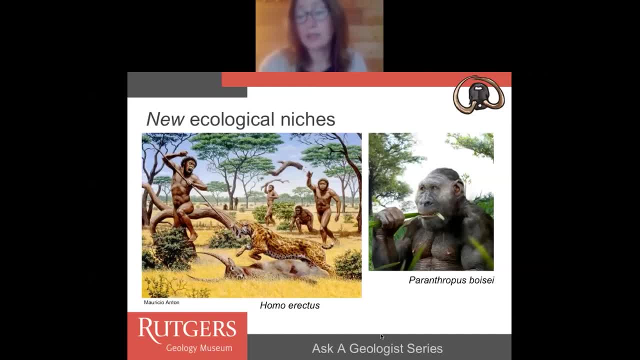 actually was a picture of competition. And so, for instance, we have new ecological niches forming. So at about, say, two and a half million years ago, when we see the savanna, ecosystems really fragment, we have a spread of grasslands, And even though the environment all looks the same, 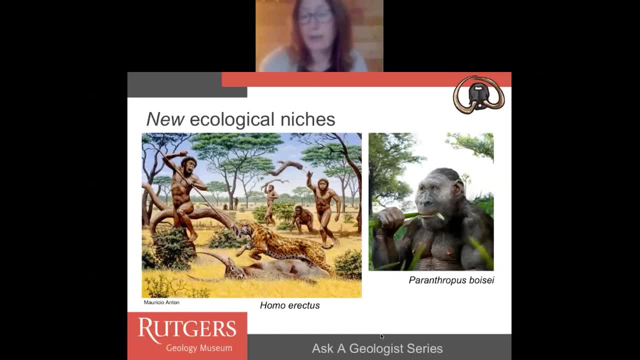 across Eastern Africa. we have both Paranthropus boisei and Homo erectus, two sister groups, these two sister taxon or two sister species living at the same place, at the same time, in the same environment, but doing very different things. And so Paranthropus. 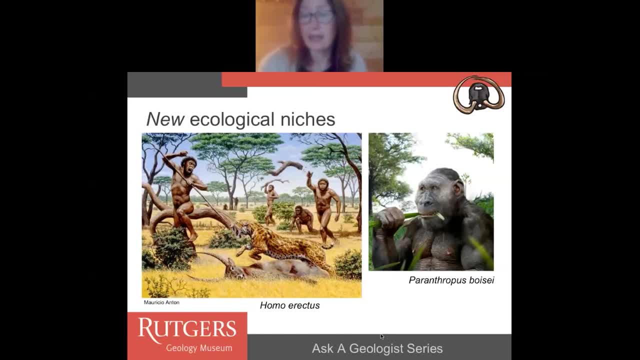 boisei is a grass specialist And it looks like it's eating grasses, grass, seeds, even potentially something like sedges that grow next to water, but eating things that are more grass, And Homo erectus is actually probably a species that gave rise to us. Homo erectus is maintaining. 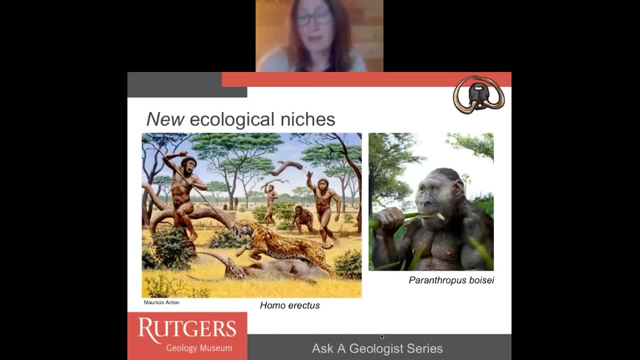 more of a mixed diet, And the diet it may have included and as this picture, this artistic picture represents, is may have been eating not just vegetables and fruits and even some grasses, but was actually eating something brand new, and that would have been meat. 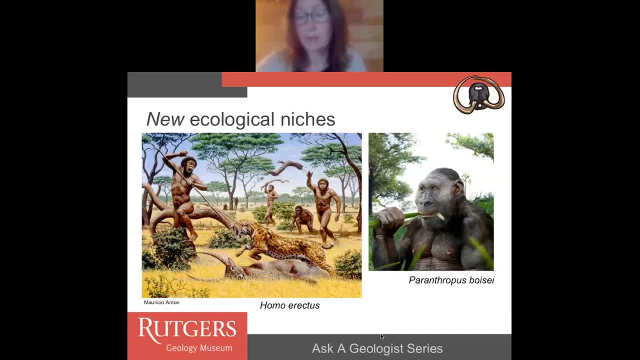 and marrow scavenged from dead animals on the landscape, And what's interesting about this time period is that would have been a time where there's competition from other predators on the landscape, And so may have given rise to what we consider a separation in the niches. 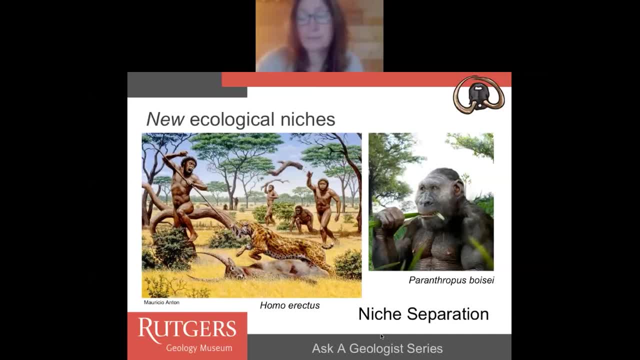 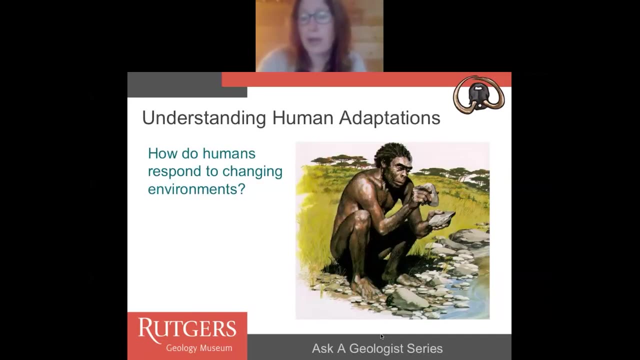 And so, even though the landscapes look the same, there's two very different types of organisms or ancient humans using those environments in different ways, And so the larger picture for us is to really understand the path, to understand how humans adapt and that we are shaped by our environments. 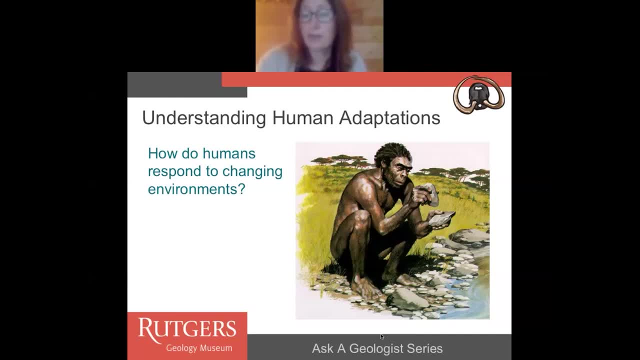 but humans themselves have a lot of things to change. They can evolve in different directions. It's not as if there's one path. There's been many different paths, And that's the part why our tree is so bushy is that we ask that question. 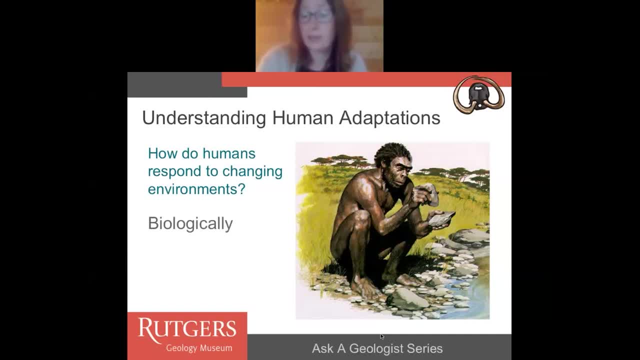 do they change to environment biologically- And we think that is the case- is that indeed, we get a bigger brain, we get a bigger body size. A part of that is living in these environments and that's a biological response to environmental change. 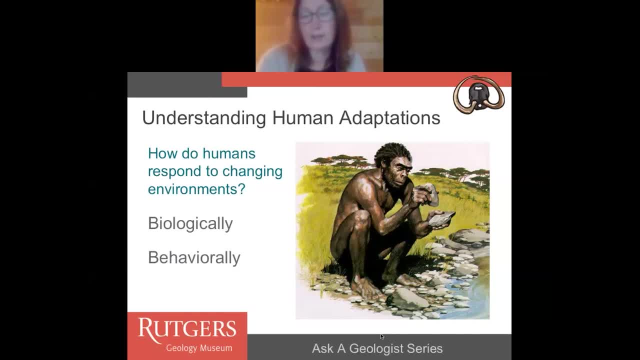 We also see changes behaviorally. is that with changes to diet, that becomes a dietary selection, a dietary preference, that different groups of humans are trying on different behaviors, different ways of foraging, different ways of getting their calories every day? And then this is an interesting point. 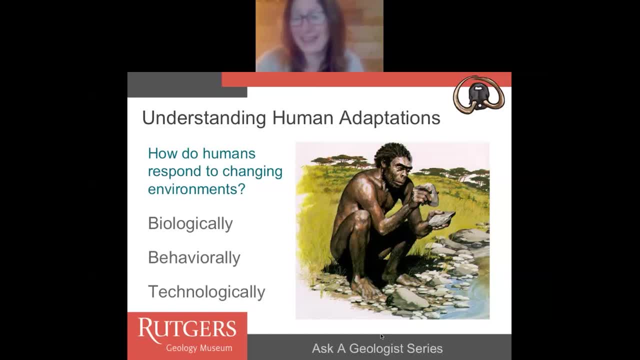 especially good, now that we're all using our technologies on a regular basis, is that from the beginning, from early on, early, early in our lineages, we start to kind of have solutions to problems, both kind of environmental problems, but also just larger problems of going. 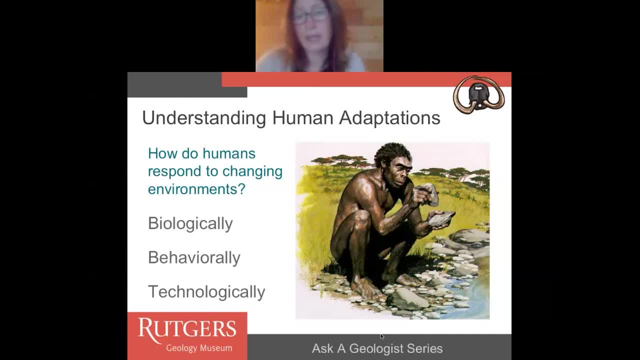 how do I get my calories? every day, We see the beginnings of stone tool technology, And so this is where ancient humans really do something that's quite different than other organisms- At least they do it a lot. It's some other organisms. some other organisms use tools. 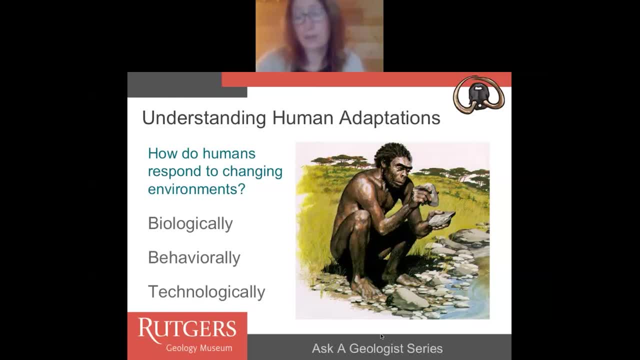 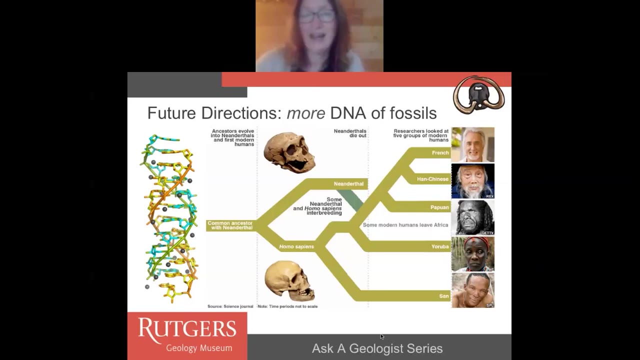 We know even monkeys have some. there's some anecdotes about tool use, but humans start to solve many of their problems with tools and with making. So I think, when it comes to future directions, there's a lot technology can help us to learn about our path. 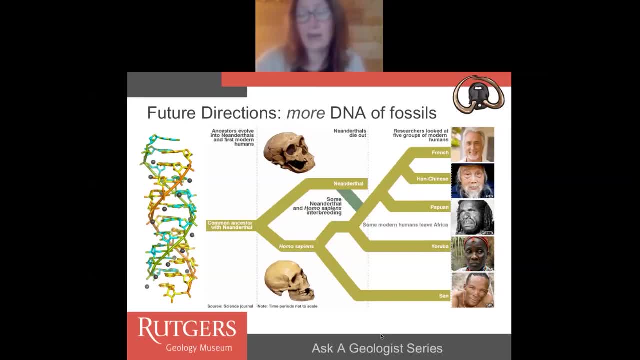 And one of those things is DNA. Now, I started by saying we do have a lot of DNA sequenced from chimps, from other apes, from modern humans, And now over the past really 20 years, we've been getting DNA actually extracted from fossils. 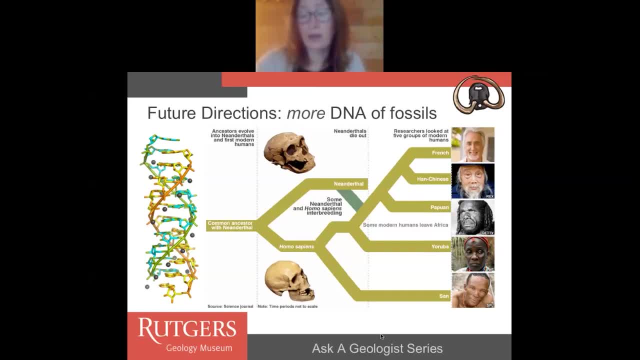 And so right now, what we have characterized very well are ancient humans called the Neanderthals that lived in Europe, and also modern humans about the same time period, And we have a sense of how that tree looked because of DNA. DNA is our line of evidence to understand. 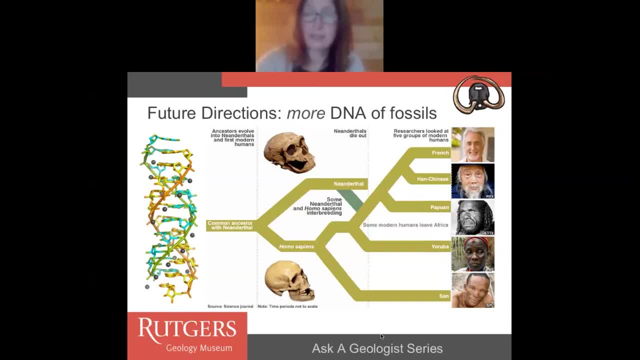 were they interbreeding with one another? Were they two different species? Future directions may reveal more DNA from fossils that extend a lot further back, And that really is a technological solution that we need to have, with better ways of characterizing DNA. Okay. 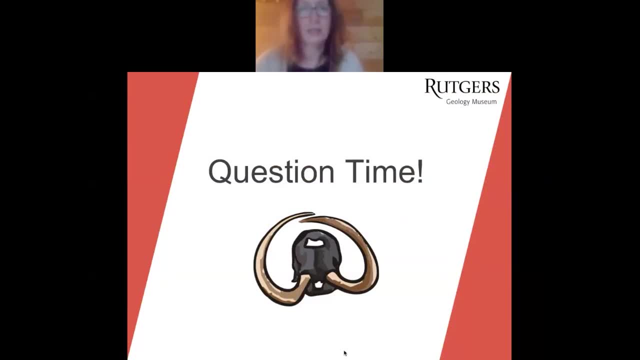 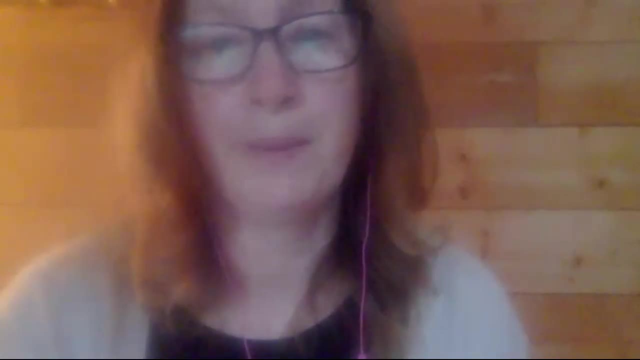 So thank you very much for listening And I will answer some of the questions that I can pull up quickly. We had a question from Madison, from Flanders, New Jersey, And the question was: would you like to know if people had- oh, people had- tails, and how long were they? 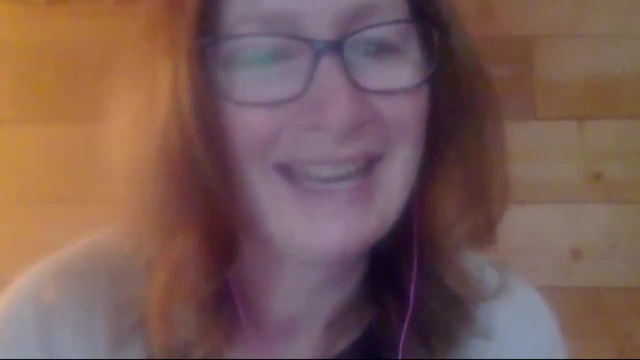 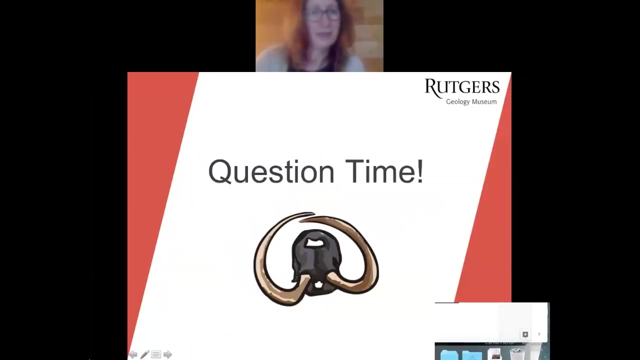 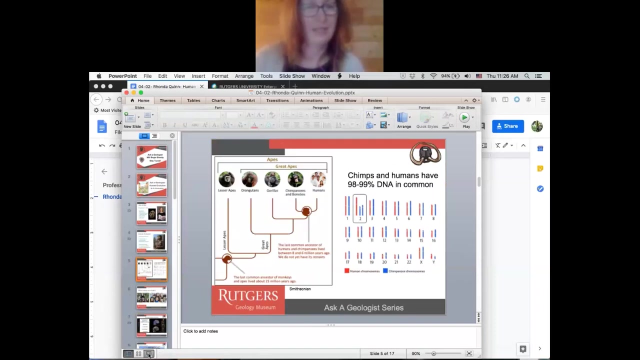 That's a great question, Cause I especially see kind of shows, cartoons kind of saying something of the sort. So I'll show you on the screen This picture- let me just go back This picture with the last common ancestor of monkey. 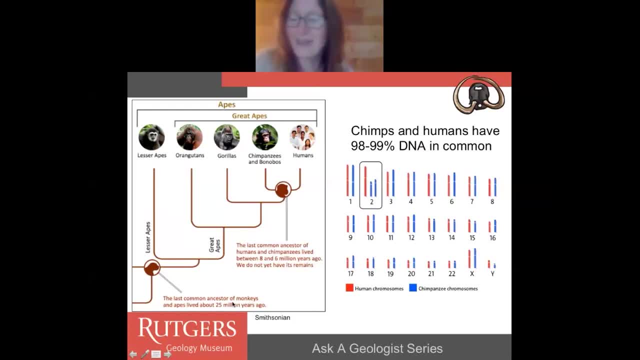 So, as it turns out, neither humans nor apes have tails, So we've lost those. So we had, and those tails are just an extension of the vertebrae. they grow in the same way vertebrae grow, or the backbone. 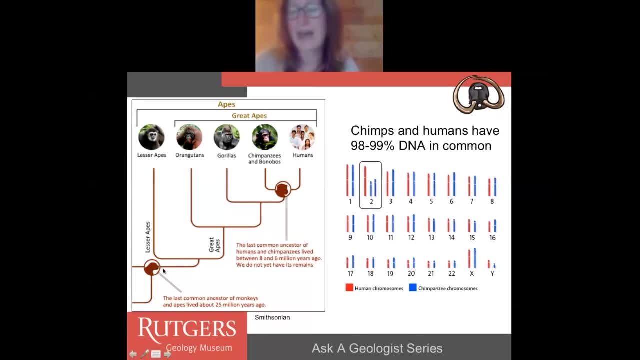 So the last common ancestor of monkeys and apes- and you can see here, it's about 25 million years ago- And that would have been the, basically the loss, so to speak, of the tail. And so no apes have tails, and neither do we. 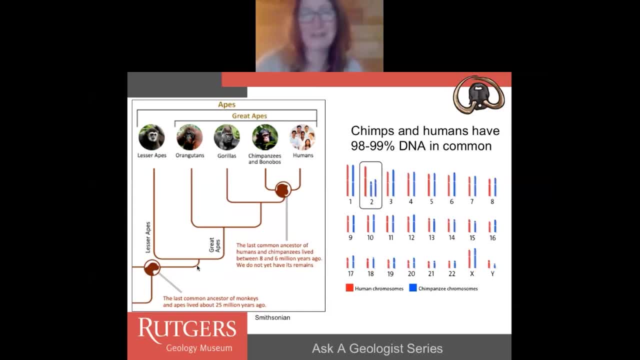 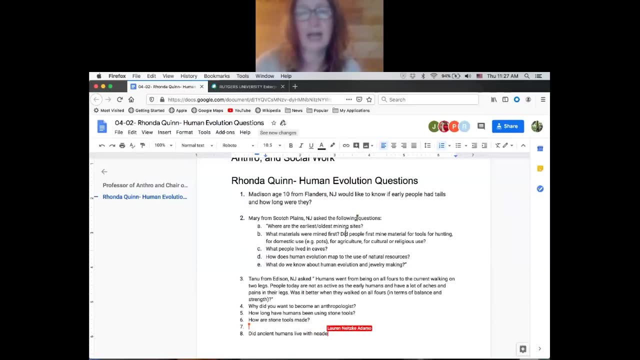 So it would have been about 25 million years ago that we lost our tails, so to speak. Let's see. Mary from Scotch Plains, New Jersey, asked the following: where are the oldest and earliest mining sites? That's a good question. 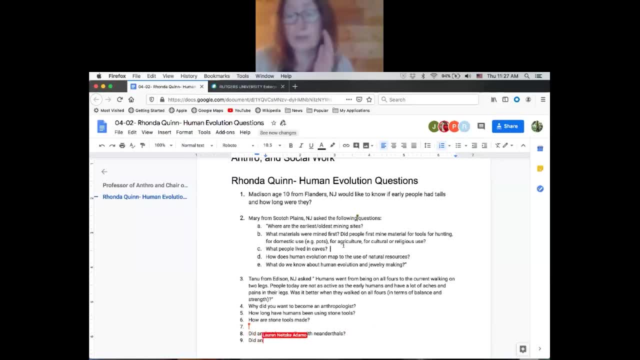 So when we think about mining, we think about raw materials that were then gathered to then either make tools or other things. As it turns out, this spans a very long time period. So first basically finding raw stone and then shaping the stone to make a tool. 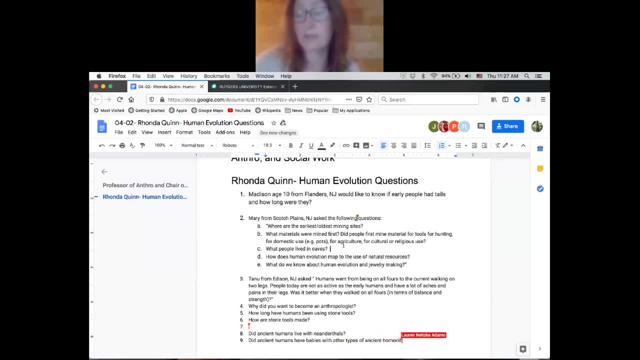 We think that goes back a very long way. The earliest evidence for stone tools comes from Kenya, in a place called Lomekwi, and that has been dated to 3.3 million years ago. The question also talks about other things like for hoth, agriculture, cultural and religious use. 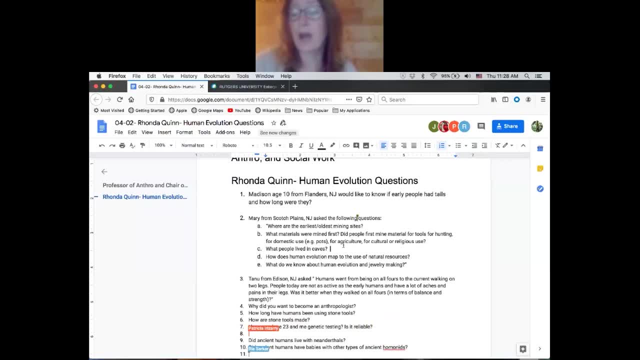 That happens later on. So we would think of pottery or ceramic. pottery or ceramic. Hey, Rhonda, Yeah, Can you stop sharing your screen so they can see your face bigger? Sure, That's fine, thanks. So pottery or ceramic would have been much later in time. 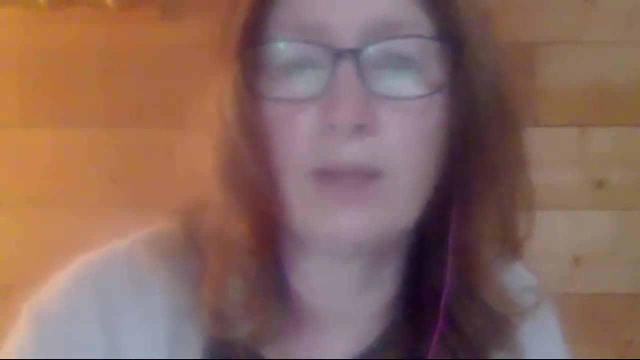 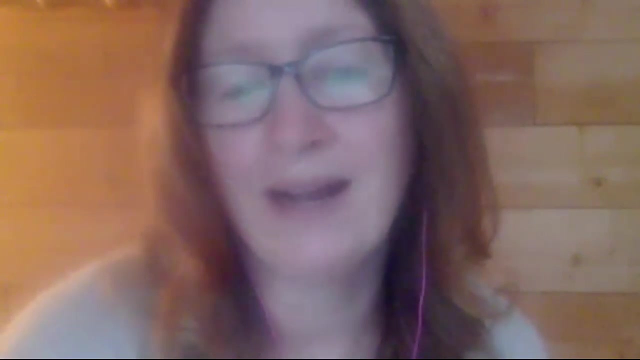 So the earliest ceramics really go back to making what are called Venus figurines. They're figurines of women. That goes back. we have some in Europe that go back about 25 to 30,000 years ago. So then pottery used for more agricultural purposes. 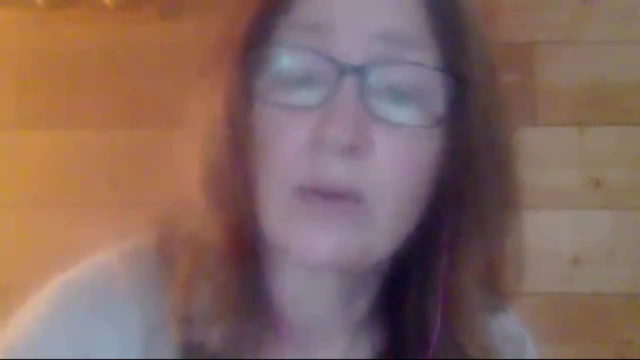 That would have been on the order of the earliest agricultures about 12,000 years ago. People widespread use of agriculture is between kind of 7 and 5,000 years ago when it becomes very global, So that would have been when people were mining of the sorts. 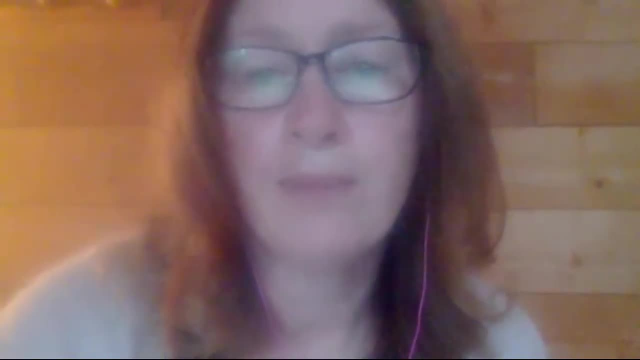 or gathering material. for that way Let's see What people lived in caves. That's a great question. So really we don't see extensive use of caves until what is about a million years ago in Europe, mostly in areas that are cold or have cold time periods. 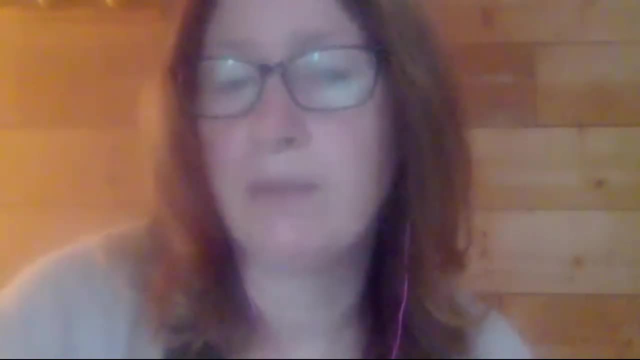 So, living during glacial periods, We see people, Neanderthals, what are called archaic homo sapiens. So about a million years ago, two more recent times, people indeed lived in caves, The earliest hominids that we have. 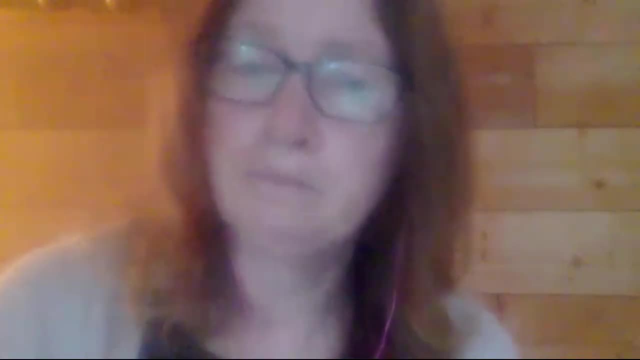 we don't have evidence that they lived in caves. They're probably living more. we're talking about the earliest bipedal hominids, like the Australopithecines. They're probably not living in caves at all. They're probably living in very much the same ways. as other primates do so, utilizing sleep trees. We do have some chimps that have utilized caves, but we don't have widespread evidence of that early on. It comes much later, mostly in Europe. How does evolution map the use of natural resources? 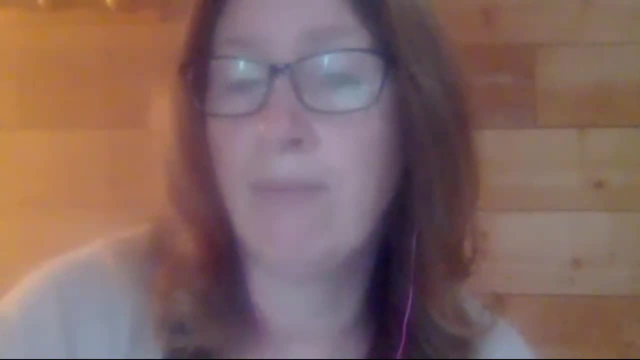 So that typically happens with understanding the materials used. So say, for instance, if you have a stone tool at your archaeological site, usually what they do is analyze the tool for the type of rock that it's used, And sometimes we use chemistry to do that. 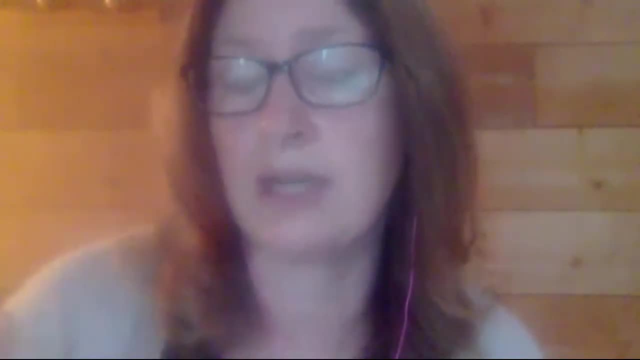 and geochemistry, like I talked about today, to characterize the rock, And then they search for the sources, and so then they map the sources And this takes a lot of walking, a lot of survey to look for those natural resources. 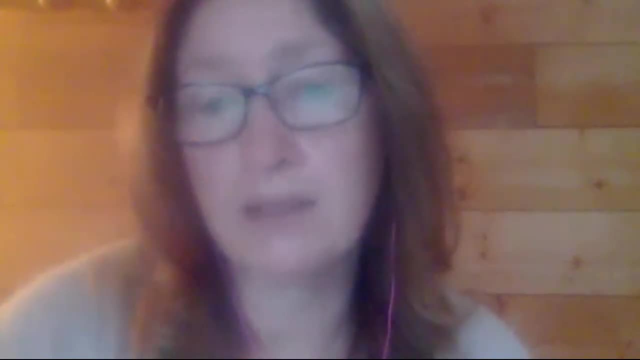 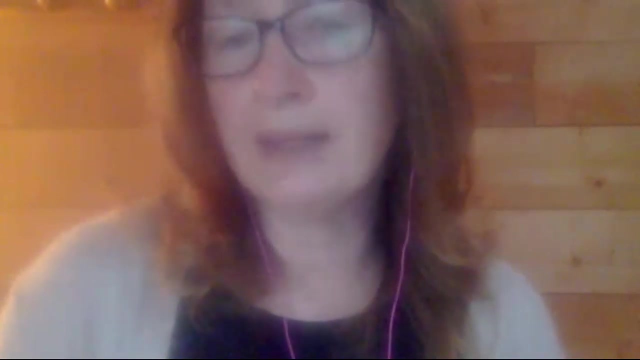 What do we know about human evolution and jewelry making? Jewelry making, that's a good one. We have early evidence of, and it's all our species. that people, I think, mostly agree upon is that it's our ancestors, it's Homo sapiens. 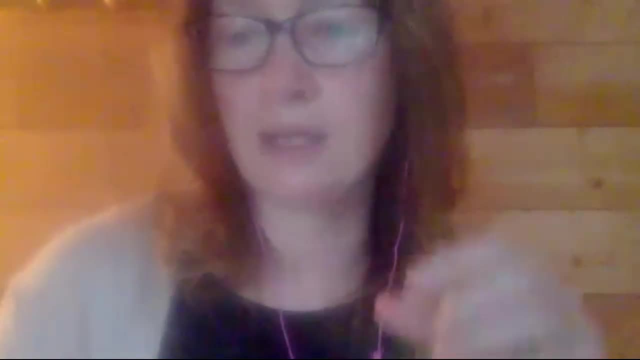 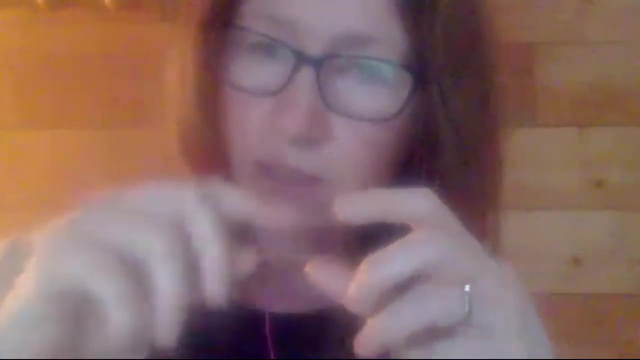 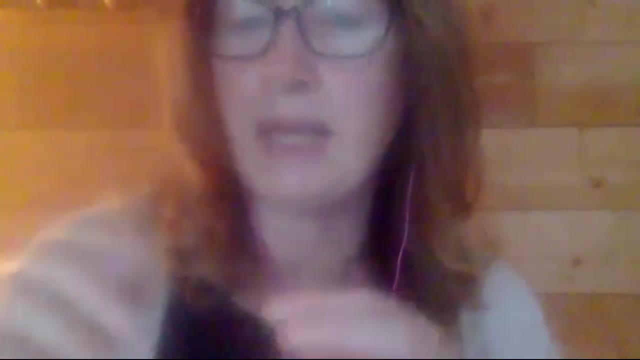 but early on that there's basically usually a shell material or even the teeth of animals, and then they perforate either the root of the tooth or they perforate the shell, And the idea is that they may be it's kind of prior to bead making. 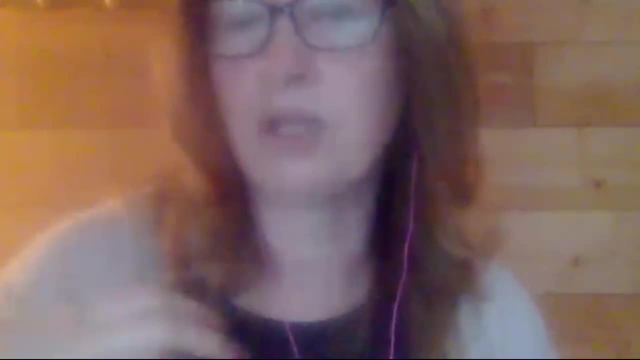 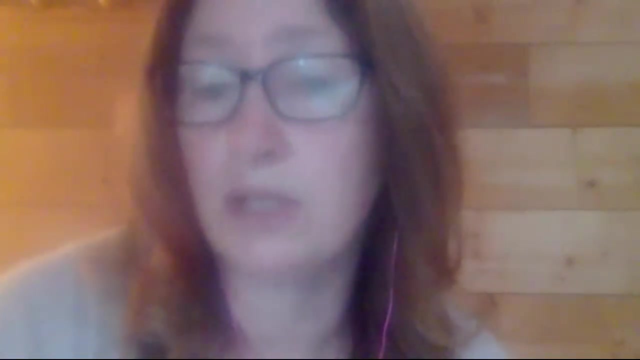 but they're probably using it to string or to sew on to even clothing and things like that as well. Let's see from Edison, New Jersey asked: humans went from being on all fours to the current walking on two legs. People are not as active as early humans. 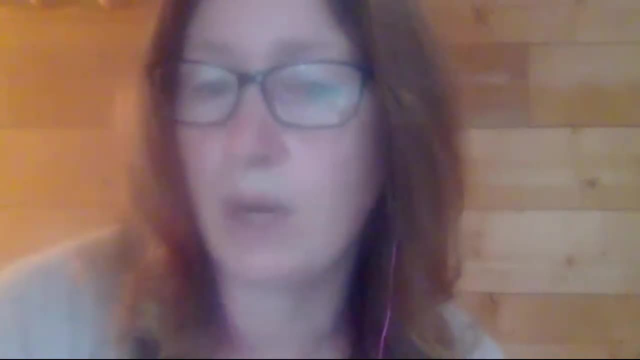 and have a lot of aches and pains in their legs. Was it better when they walked on all fours? in terms of balance and strength? That's a great question. The question about aches and pains today probably has more to do with how long we live. 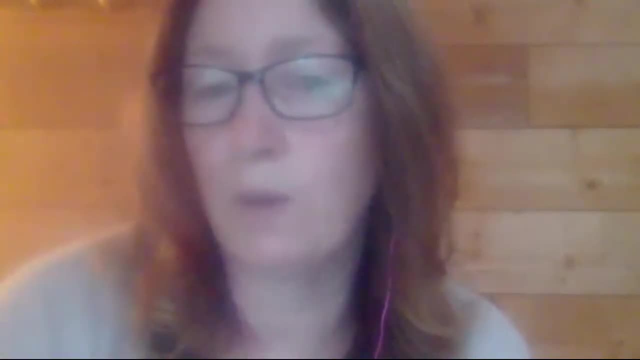 and how inactive we have become. So it's more modern that we're. you know, when we are sitting in front of our computers, it's actually the worst thing that you can do for your body And the idea that you want to get out and walk. 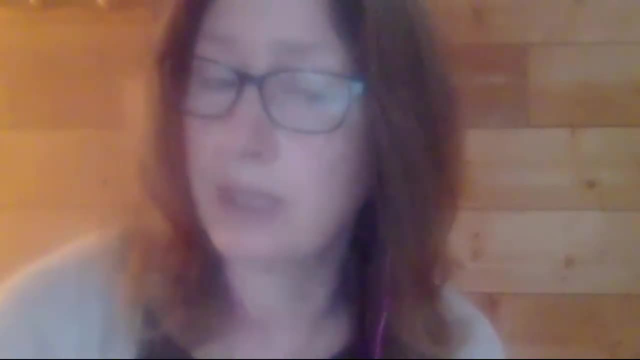 We've been selected to be walkers and even runners, So walkers, in particular our body does very well with In terms of overall aches and pains. we can, of course, have underlying conditions that are pathological, But we in many ways it is also kind of a consequence. 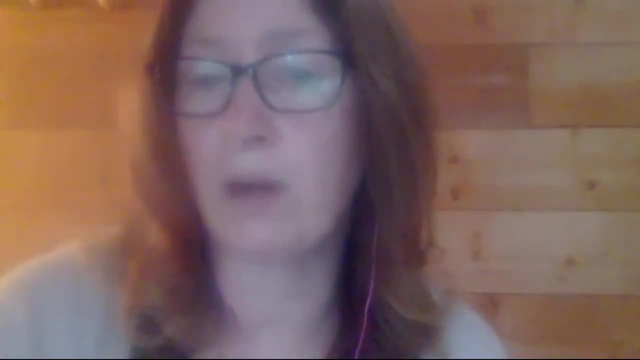 of living such a long life. You know, our body for the most part was selected to kind of go well into adulthood. But we have extended the life And we have we put extra stresses on our body. I will say there's an idea called a design compromise. 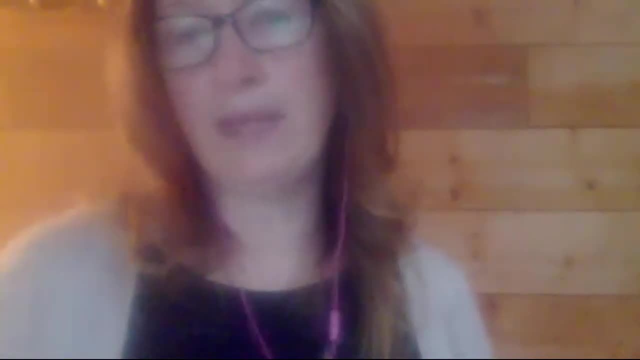 And that's going from an evolution being on all fours. Our body is selected to be bipedal, But there is a consequence, we think, in the lungs. It's a long term, not as a young individual, but as an older individual, that we do have some things. 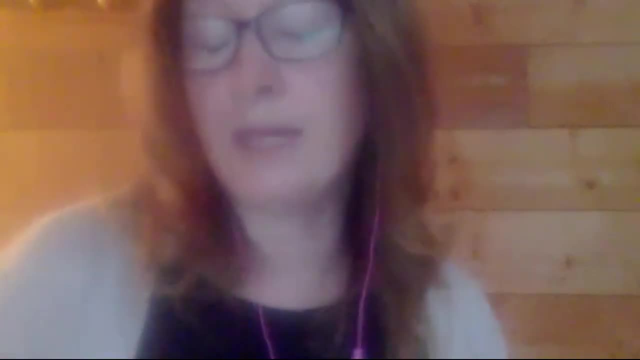 especially in the lumbar, the lower back region, The knee. the knee is not a great configuration. It's not a great architecture, especially for high stressors. So a lot of it depends on the amount of activity right Overuse can put a lot of strain on our joints. 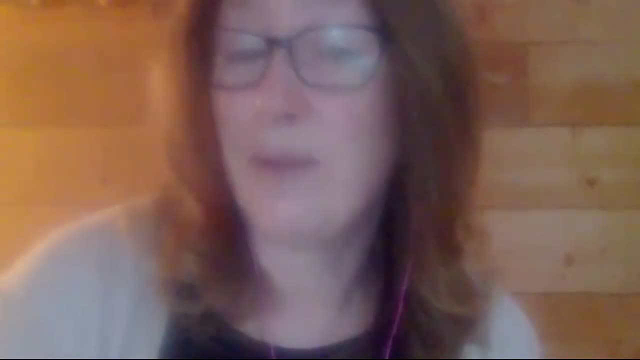 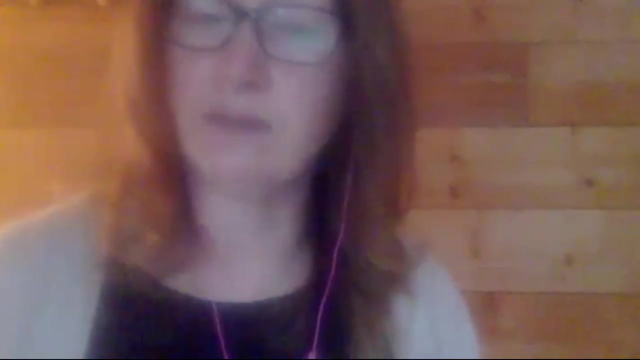 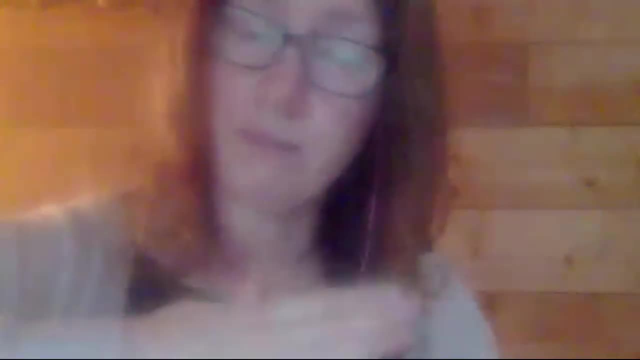 How long have humans been using stone tools? As far back as 3.3 million years ago. stone tools are made by taking. there's a few ways of doing it. You can take a rock and hit it with another rock to make a sharp edge. 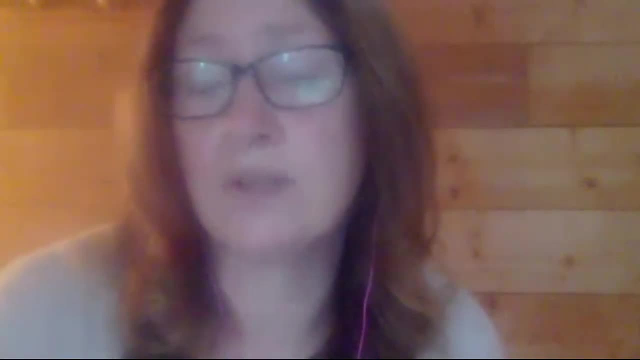 You can also take a rock and use kind of an anvil to then bash down on it. There's different types of materials used to make rocks, depending on if you're doing something. that's kind of a pounding or, you say, a percussion. 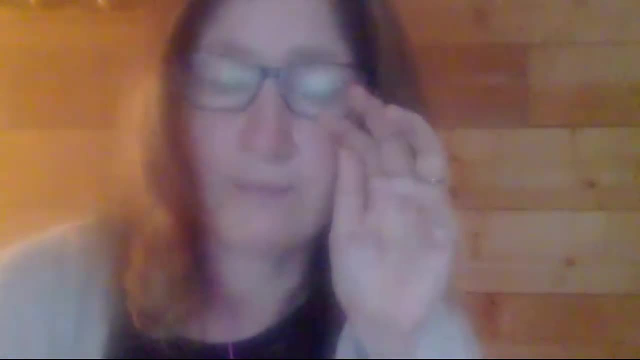 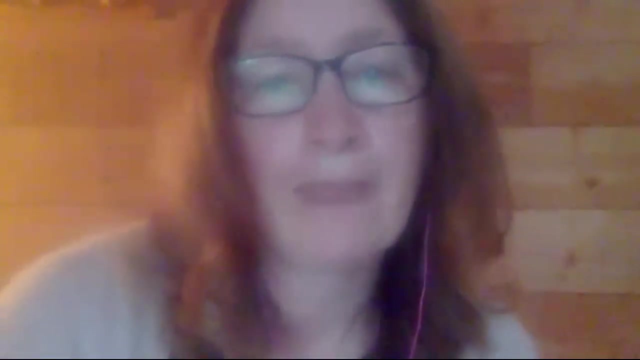 Technique or even more of a precision. So things that are you're just retouching an edge, use it in different ways. Have you done 23andMe genetic testing? Is it reliable? Interestingly enough, I did both 23andMe and Ancestry. 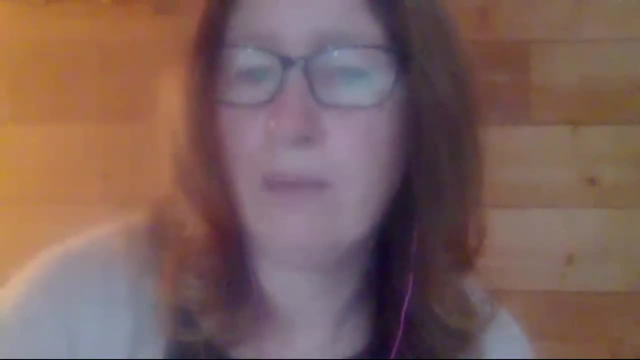 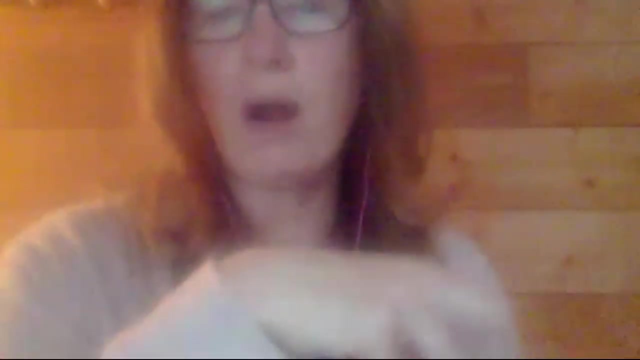 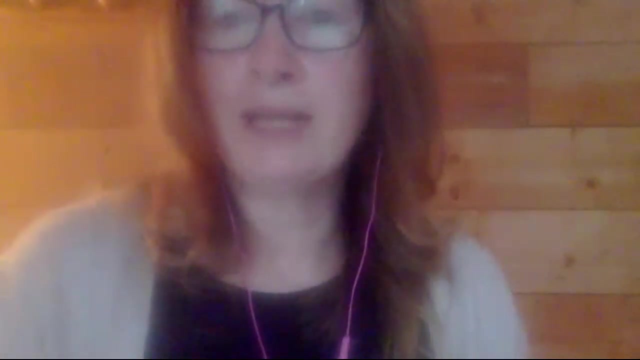 because I was interested to compare. Is it reliable? Sure, I think the biggest question is the database itself, And so the database that the group uses to kind of match where you are as an individual is all based on how much we know. And so that means because when you get measured, 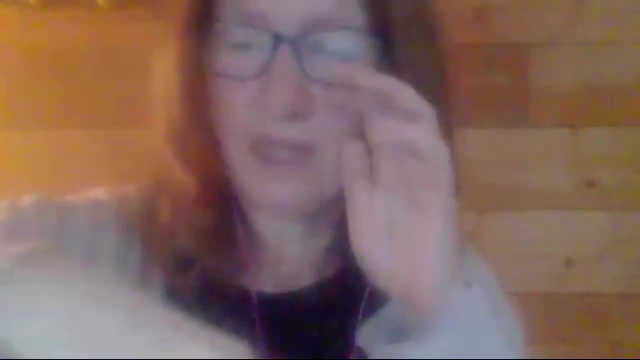 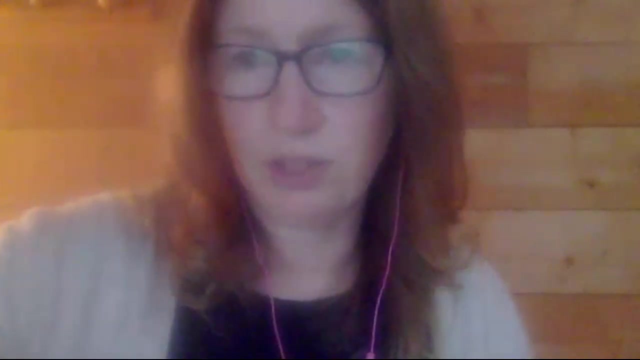 they're assuming you're kind of an unknown. They take your kinship. you know there's a lot of kind of kinship information. they ask about you. But the idea is they're putting it into an established framework of people that they have an idea of where they come from geographically. 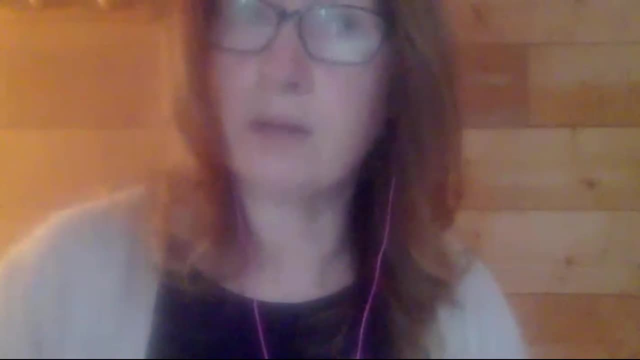 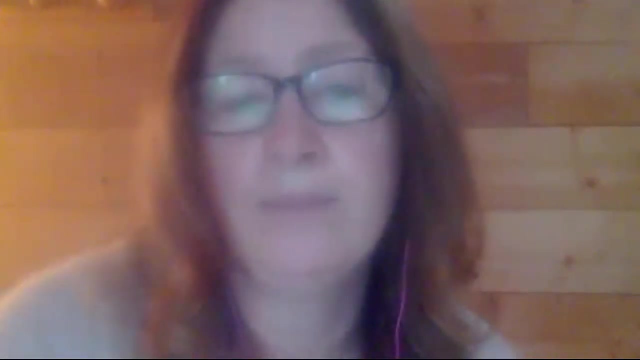 So the better. the more we characterize known individuals, the better the genetic testing and the reliability will be. Did ancient humans live with Neanderthals? Likely they lived alongside Neanderthals. There may have been some interbreeding. The DNA is suggestive of that. That ancient modern humans indeed lived in the same times and the same places as Neanderthals. They do maintain morphological differences, or what they look like. There may be some cultural differences, But that's a great question And it's still something I think people debate a little bit. 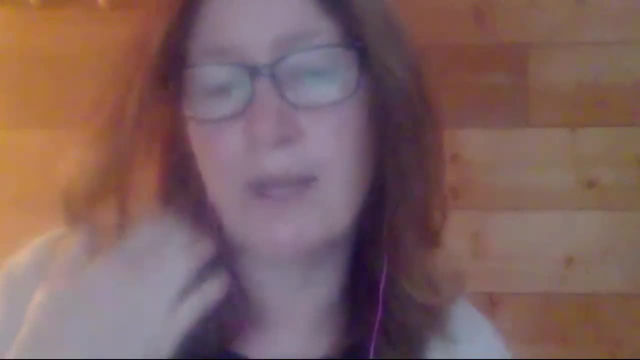 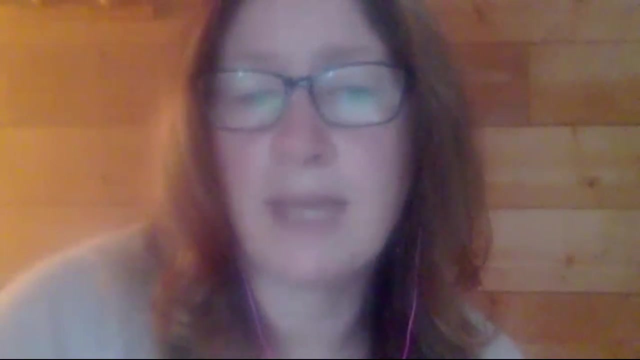 How much interbreeding. if there was a little bit they share, a little bit in common, Was there extensive interbreeding? Because anatomically modern humans, modern humans- do show some differences when it comes to kind of cultural differences and the things that they make. but also what they look like as well. Did ancient humans have babies with other types of ancient hominids? It would have been. that's a question of what makes a good species. That's a really actually it's a heavy question. because we have lots of evidence from modern times that things that we think are good species actually can interbreed and make a baby. that's also viable, meaning that that baby can also have babies eventually, right. So the idea is like if you put together a horse and a donkey. 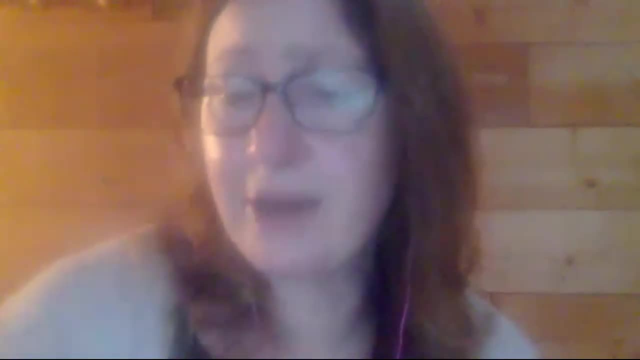 you know that makes a mule and that mule is sterile. And so we would say that you know, those are two good species, that really they can't make babies, They can make one, but then it stops at that first generation. So then the question is: well, do we have others? So, for instance, a domestic dog can have a can interbreed with a wolf, a jackal and a coyote. So then does that mean they're all the same? No, because a jackal, a coyote and a wolf cannot interbreed with one another. The same thing we would say for a lion and a tiger: They can make a liger, which is a viable offspring, So there could be a. 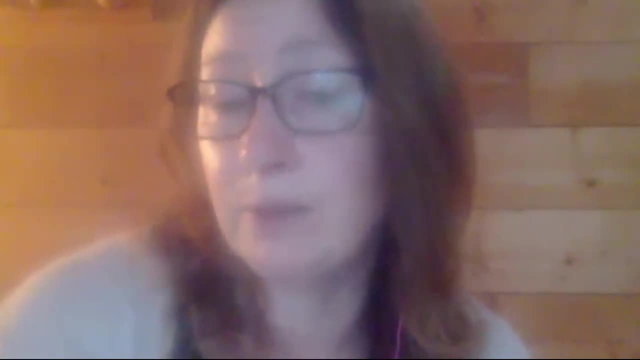 it's a larger question. We think that ancient humans may have possibly been able to interbreed with Neanderthals. Maybe the question then becomes: did they substantially, even if they could? Philosophical question: Let's see, Teeth are useful in telling us about the past. 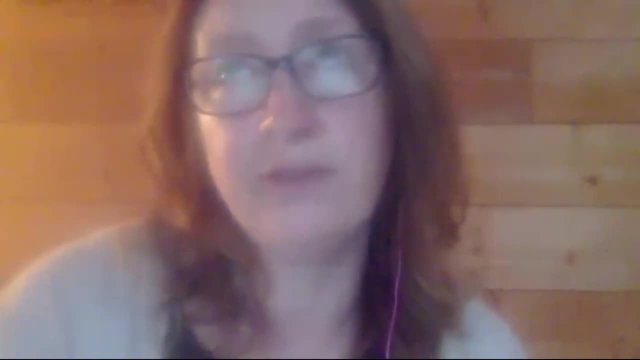 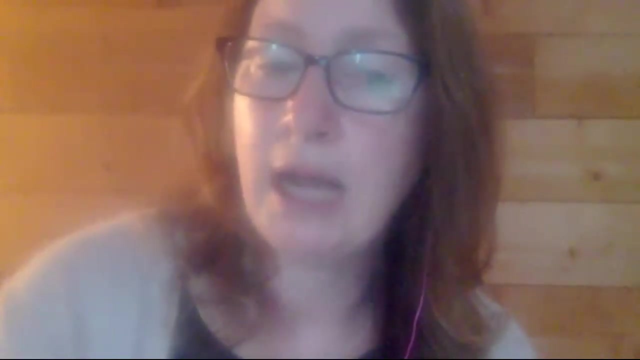 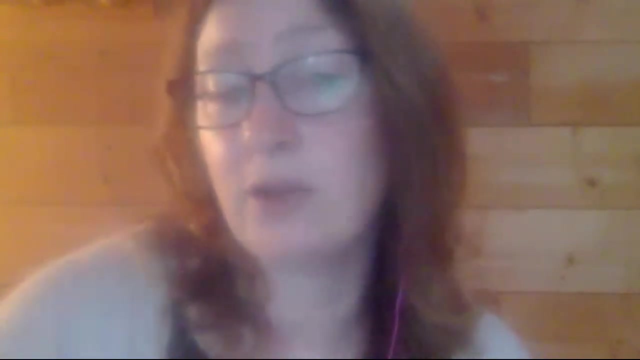 Absolutely. Teeth preserve very well. Teeth are minerals in your mouth And they absolutely tell us a lot about about difference in species. We see a lot of difference in species across the morphology of teeth. Teeth can tell us so much about what the organism may have eaten. 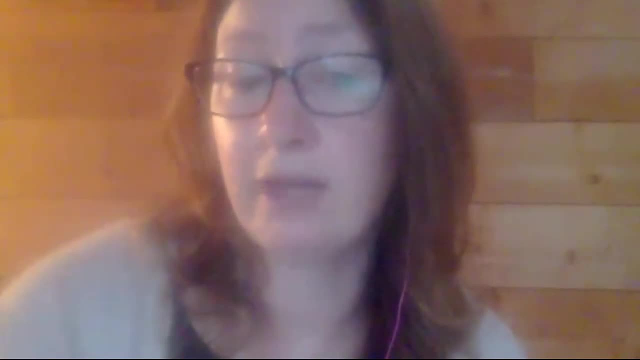 And in terms of the chemistry of teeth as well, have given us a lot. Wow, these are a lot. Okay, let's see. Paleo diet seems to be popular today. What are your thoughts on eating like our ancestors? You know, what's funny about this is that 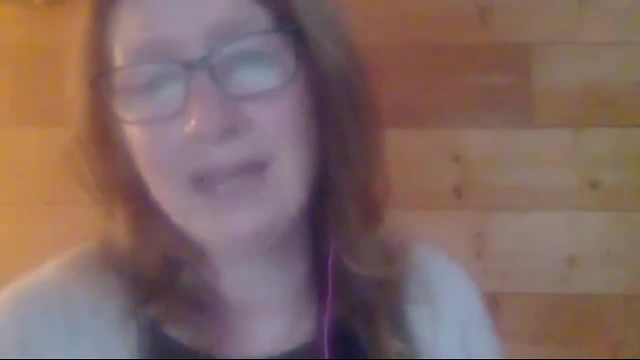 we probably eat much, much more meat than many of our ancestors, And that's because we have access. well, us is a certain socioeconomic class in the United States- have access to lots of meat. When you think about how an- you know- an early hunter would have lived. 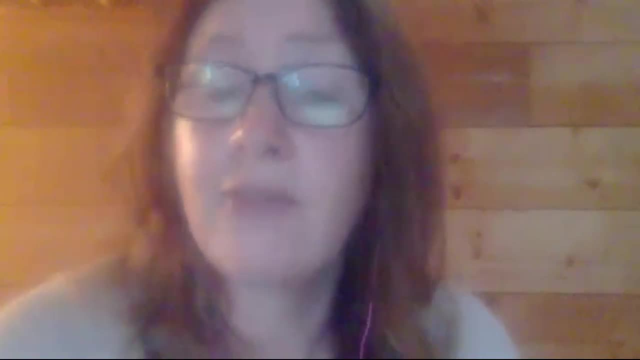 chances are- and we know this from a modern hunter-gatherer population- meat is not going to be the main portion of their diet. They would have eaten lots of vegetables. So I think, in terms of overall diet, our bodies for a long time. 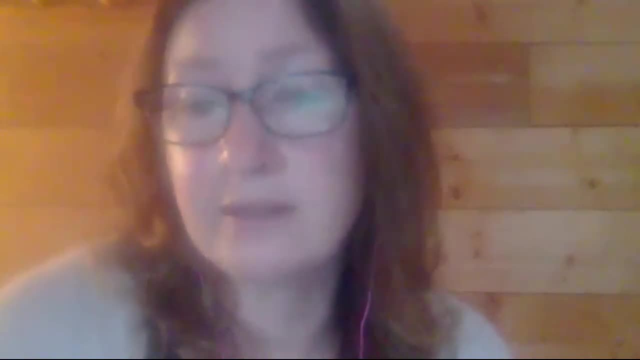 have been eating lots of leafy greens, lots of fruits. That seems to be the biggest piece of the diet. that meat is absolutely, as a protein component, is a very important component. But people, I mean I guess the biggest thing I would say. 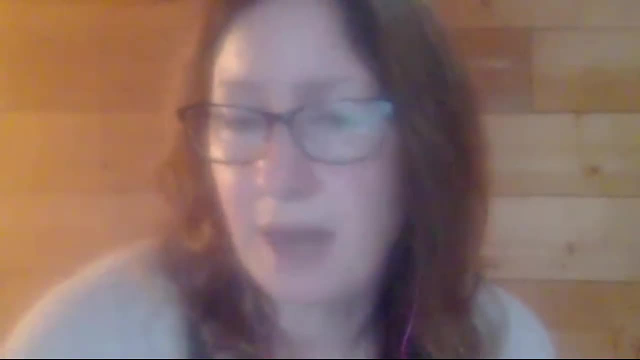 is that people all across time and cultures have made lots of different diets work well. I think the question about diet today is that we are in an industrialized use of diet And we know we know that a lot of the industrial use 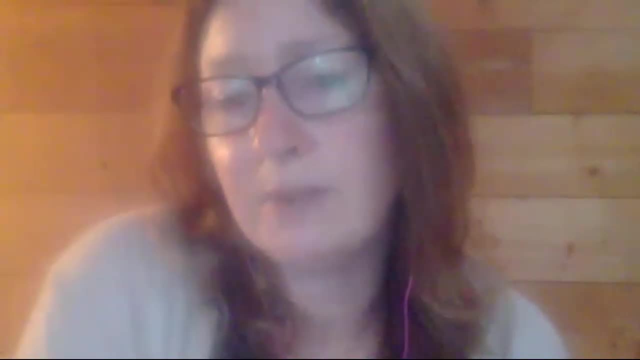 what happens to our sugars? they're refined, we have too much sugar, we have too much fat impaired, and then we don't exercise, we don't walk. Those combinations seem to be not good for our overall health. Is carbon dating used in anthropology? 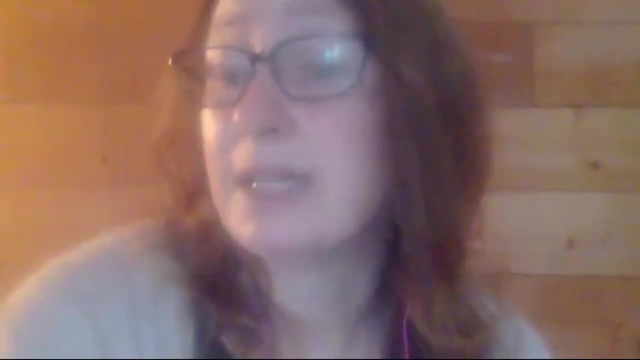 Yes, it is Carbon dating, so it's carbon 14, is the actual element It can be used. it has basically a window of time that it can be used. We can date more recent things, but it's about 50,000 years ago. 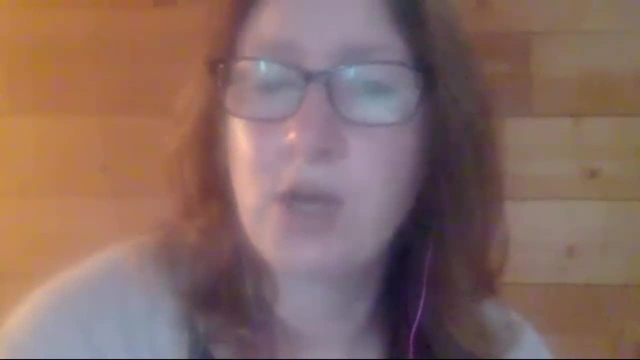 is how old it goes back, And so, in terms of fossils, carbon dating doesn't doesn't help us. We use other types of dating techniques that are the based in the same radioactive decay of elements, And that is something that we typically 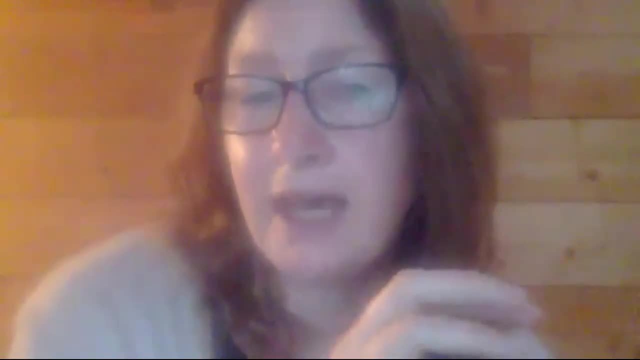 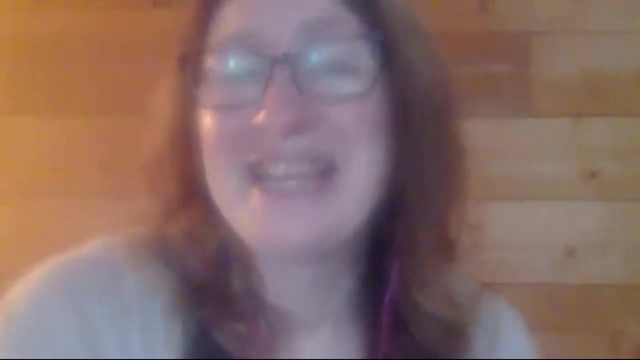 we actually measure the sediment that the fossil is found in, rather than carbon dating. that actually dates organic materials, the bone, shell, things like that. How did humans get to all the continents? You know, that's a great question. There's different time periods. 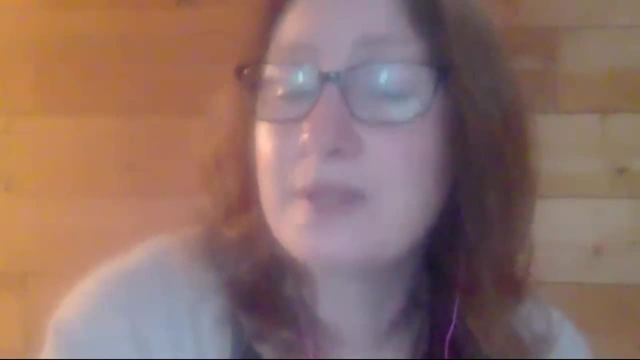 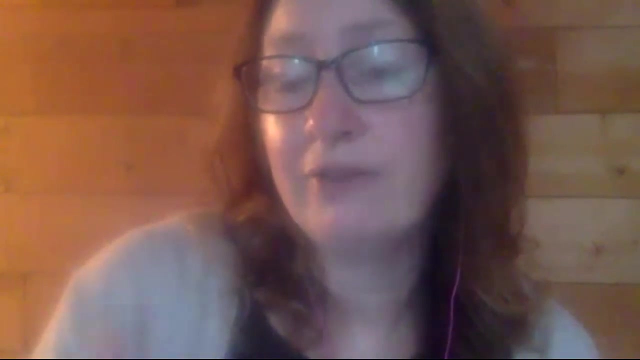 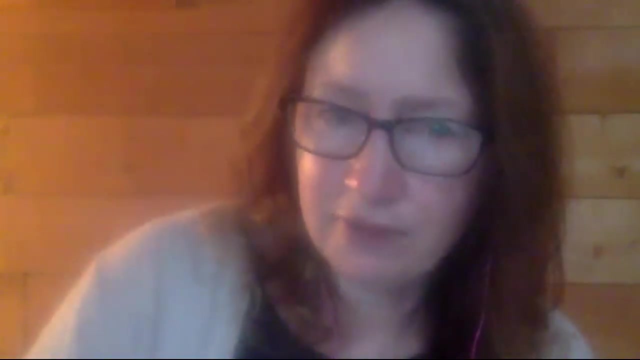 and different kind of avenues. Mostly, we think that people are living and they're ranging into areas that have land, bridges or that just have sea levels fall and come up and as sea levels fall we get a lot of land that's exposed And I think, by and large, 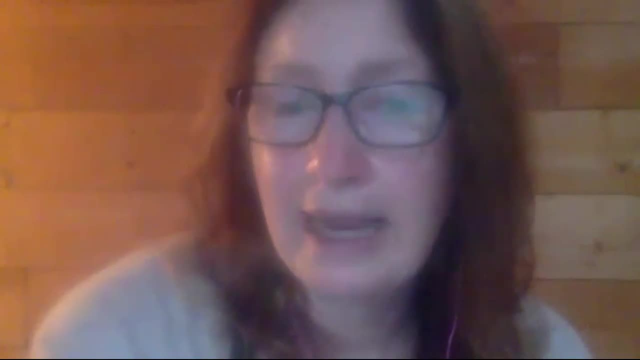 humans are moving across continents, across land. It's not to say that in later times that they didn't have watercraft and things like that, But by and large we think most human history is across land And that people aren't necessarily. 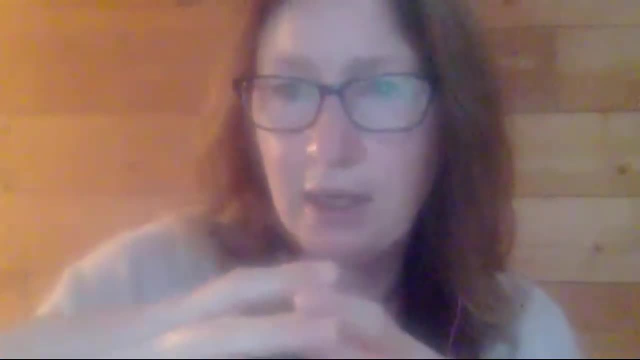 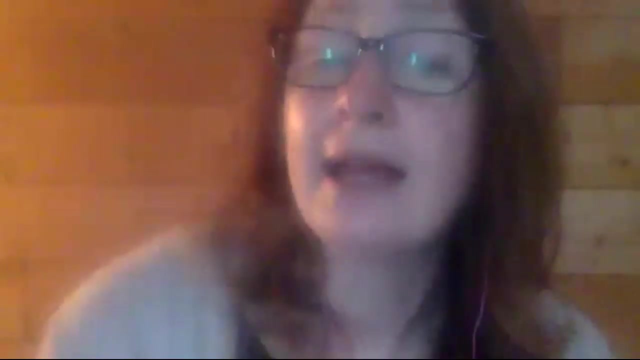 you know, packing up their bags and going. They're just living and looking for food and ranging, And as they bump up to other groups, they might move into more distant environments from where their original source was. Did early humans use animals or have them as pets? 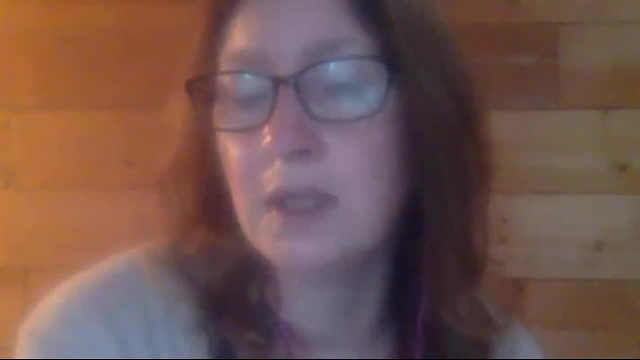 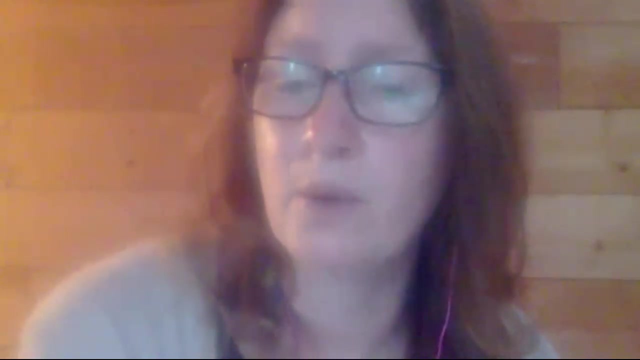 So the domestication of dogs. there's actually a lot of research on that. That's probably the one of the earliest pets that we, or we call them right. There's not in the same ways that we treat them today. more like, but absolutely humans and dogs. probably on the order of 20,000 years ago, humans have been living with dogs. There's some early burials of dogs and puppies in particular with humans. But that's yes, there's been a bit of a. 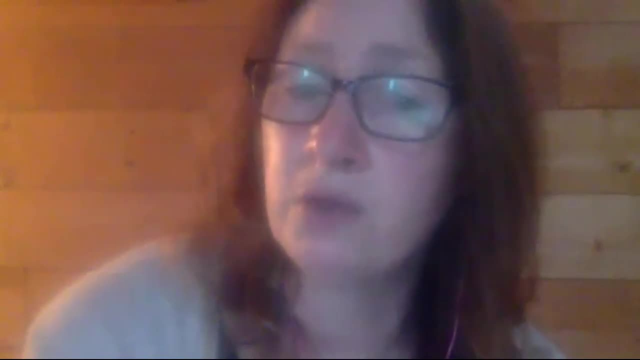 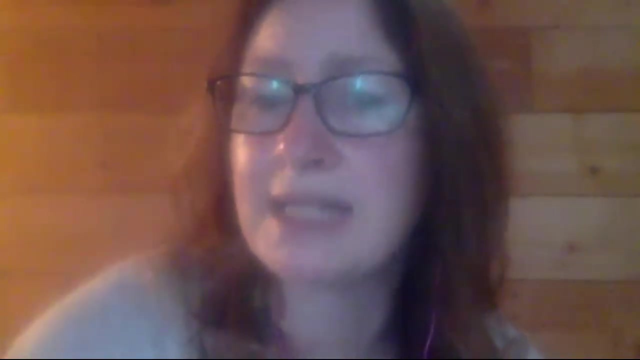 what we think a co-evolution between humans and dogs for thousands of years. Do you think that hair, the hair that early chimps had, protected them from solar radiation? Absolutely, I think that that's one of the ideas about one of the ideas about becoming bipedal. 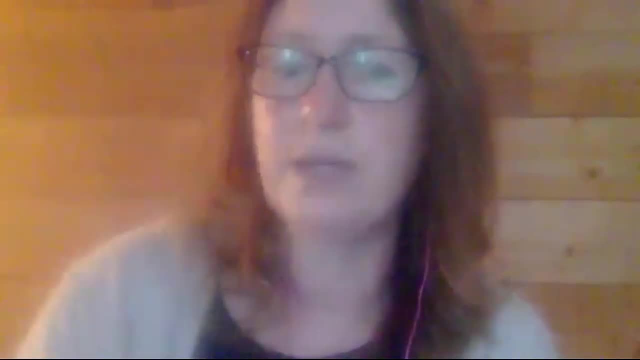 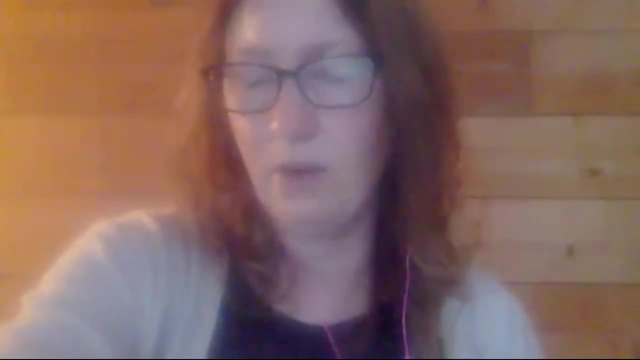 and maintaining hair on the top of your head is that it absolutely does protect from solar radiation. There is, and if you, if you kind of look at how much hair you have, it's not wholly different from how much hair a chimp had. 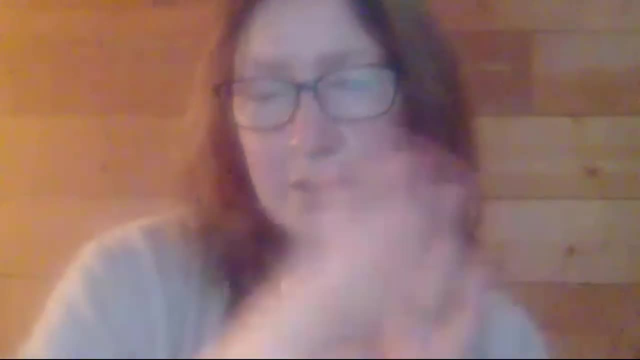 It's the. we have little bitty wispy hair and of course there's variation, But the idea is that we actually give up a lot of our hair to sweat. There becomes a trade-off of kind of how many sweat glands we have. We reduce the amount of hair so we can spurt that sweat. But then we then have a quick, a quick- actual- at least we think it is quick- selection for skin color. So the pigment in skin becomes a protection from solar radiation. 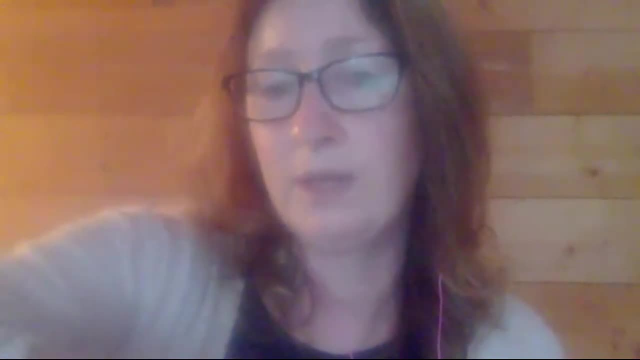 at the, at the tropics, And that we then quickly change the skin pigment and the amount of skin pigment we have And we evolve different skin pigments in different areas that, by and large, just show where solar radiation is and isn't across the globe. 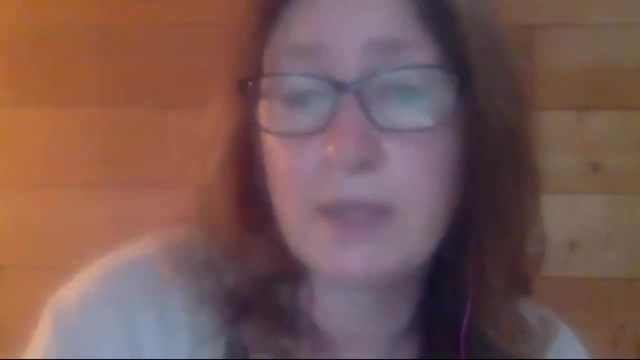 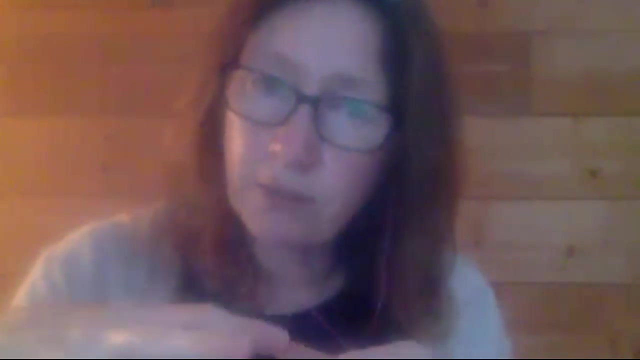 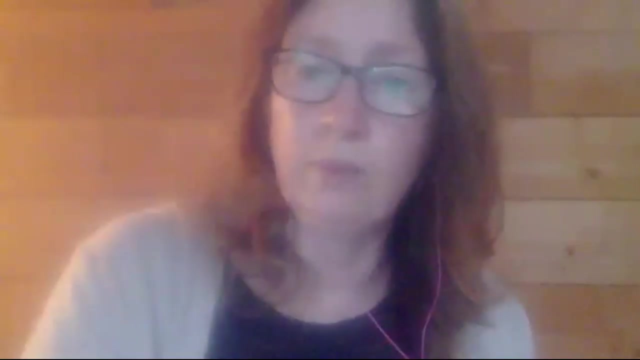 Why are so many early humans found in Africa? We think that because our origins are in Africa, That both from the origins of our lineage of the bipedal, so from the earliest bipedal hominids, we think that evolution happens in Africa. 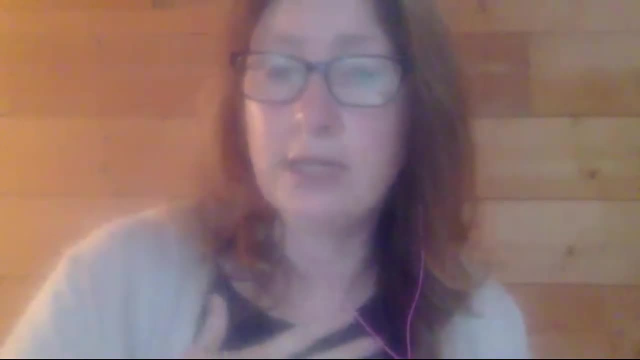 The earliest members of the genus Homo are a genus, so about two and a half million years ago That happens in Africa. And then Homo sapiens- modern Homo sapiens- originate in Africa about 200, 300,000 years ago. 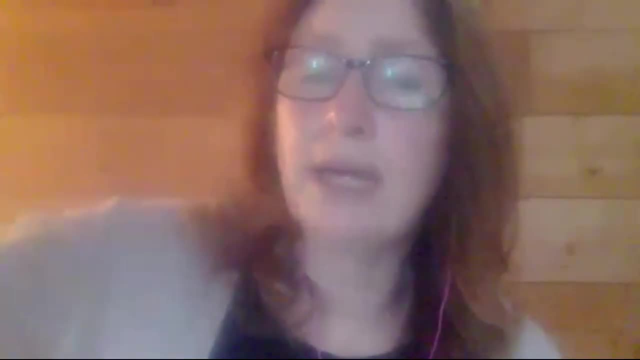 There may be some groups around the circum-Mediterranean as well. There's some more newer evidence about that. But we're not talking about a geopolitical, it's not a, it wasn't a country. We're talking about kind of landscapes. 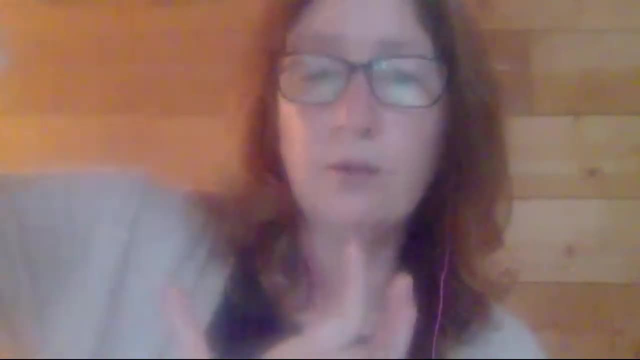 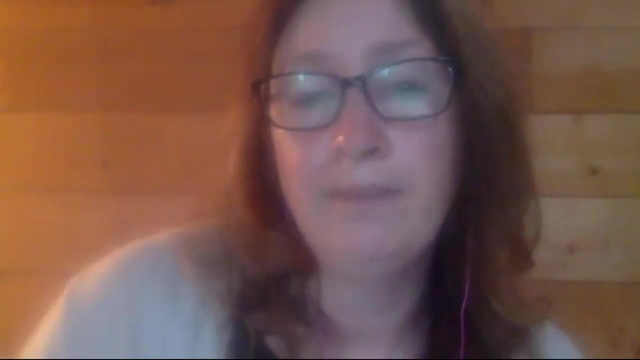 and environments And where early humans were selected to be bipedal, selected to have a big brain, selected to have this kind of tool-using way of life, And Africa seems to have the environments that do that And later on in time, 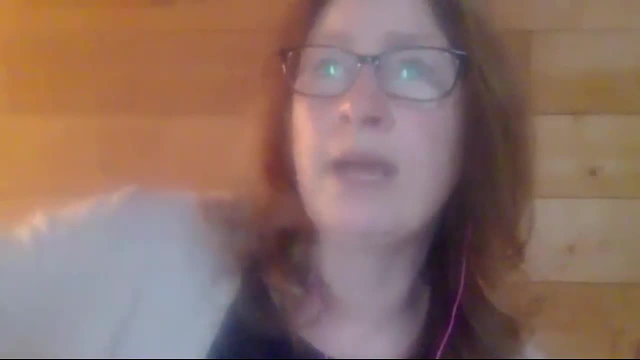 from about two million years ago on onward. we know Asia and Europe are also a part of that And that humans disperse- disperse in and out of Africa, But there's movement across what we would call the old world. What types of foods did humans eat? 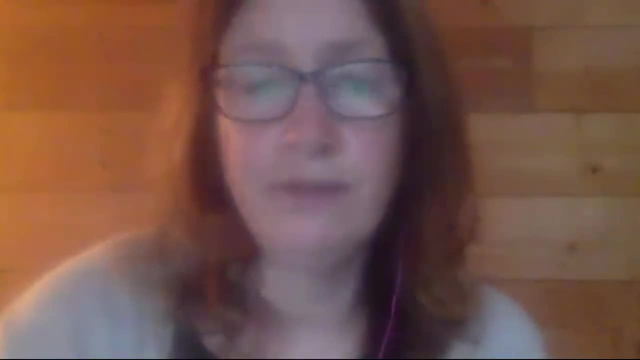 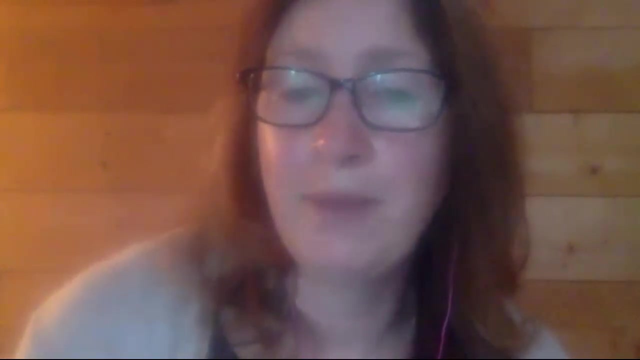 Meat and marrow, Definitely, But also, we think, more of vegetation. So what's, I guess, maybe the best answer for that question of what types of food do humans eat? Humans can eat just about anything. They have an amazing ability to be omnivores. 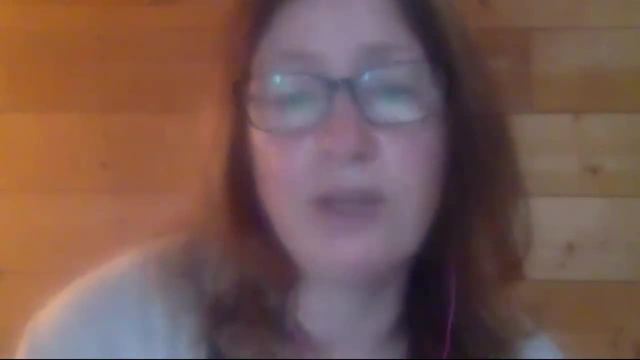 and make calories work. in many different configurations. Did early humans farm? We don't get the rise of agriculture until about 12,000 is some of the earliest evidence- 12,000 years ago And it and then we have kind of widespread agriculture. 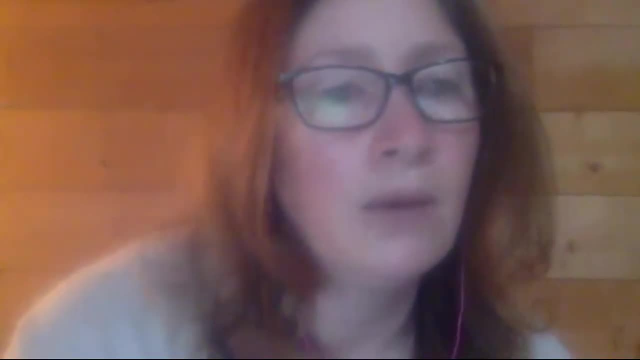 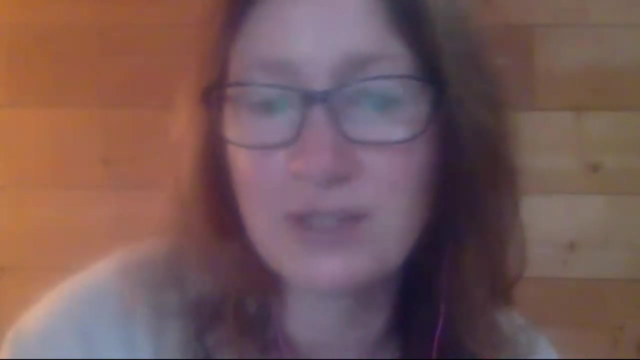 between about five and seven. Okay, So I think that all of the questions which was: oh, that's good, Everybody's really excited about this. So I'm, I think, thank you for coming, I think, I'm, I think I've finished up.